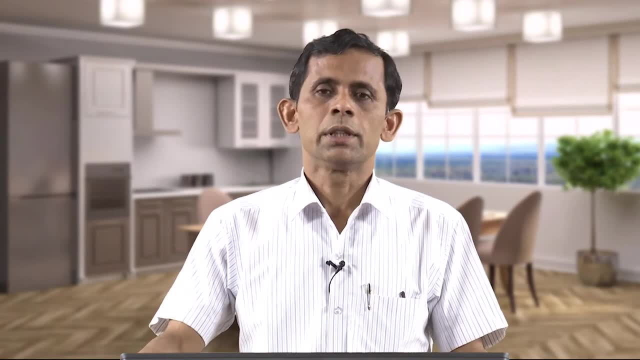 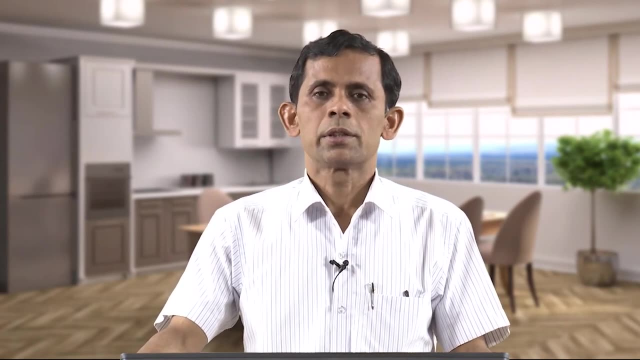 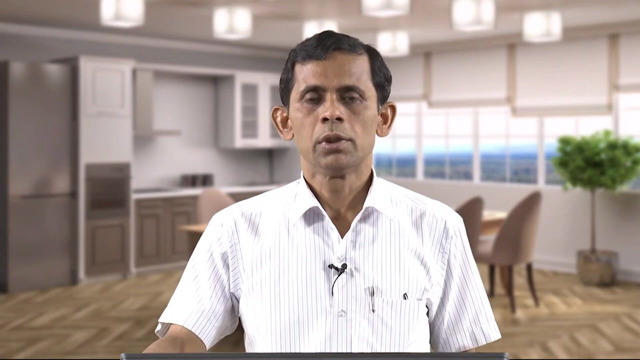 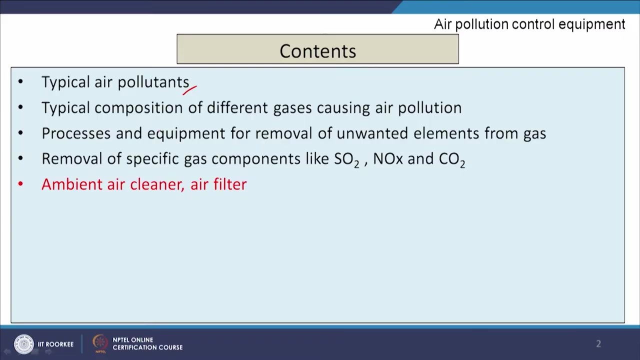 care. So in that case, what pollution is generated? that has to be controlled and this can be done by using different equipment and instrument and different methods. So that part we will discuss in this module and the contents are: typical air pollutants. typical composition. 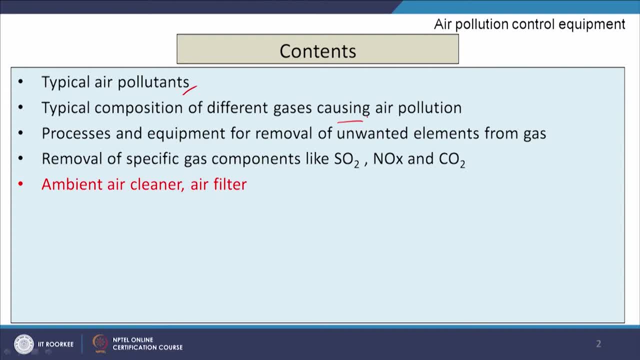 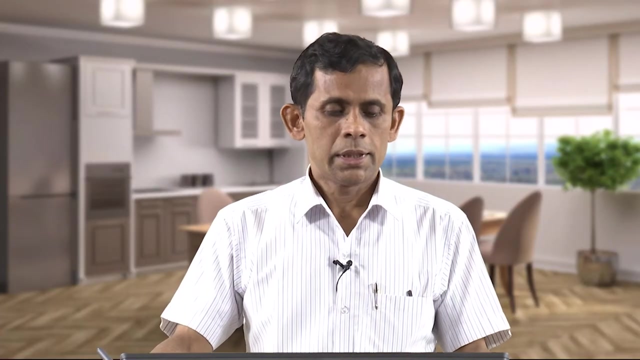 of different gases causing air pollution. So the first part we will discuss is the removal of unwanted elements from gas, removal of specific gas components like SO2, NOx and carbon dioxide, and ambient air cleaner and air filter. So this content we will cover in four classes. Now we will see typical. 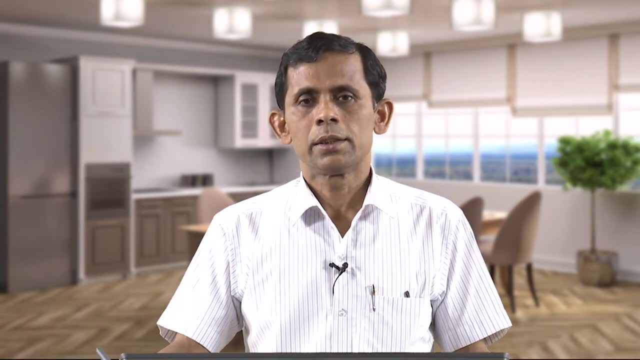 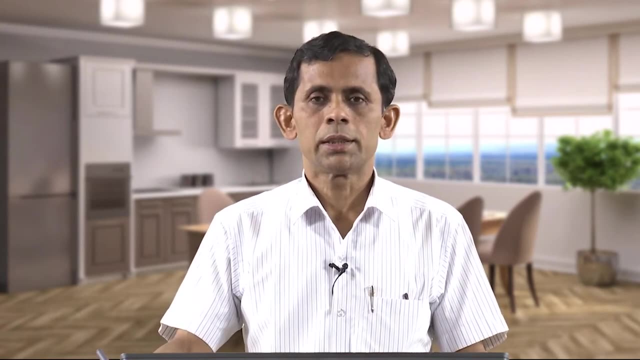 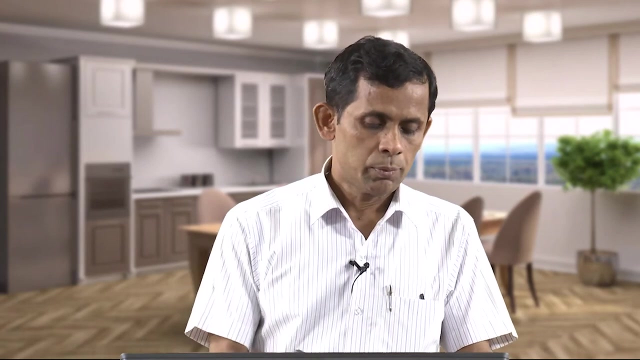 air pollutants. Already we have discussed that there are number of criteria- pollutants- which are very, very important for the quantification of air pollution, quantification of air quality. those are particulate matters, Sox, Nox, Ozone, Lead, and apart from 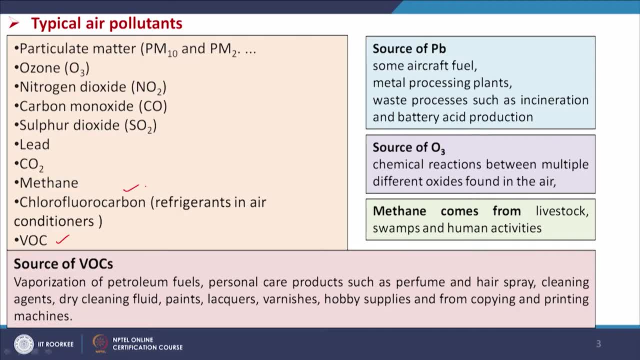 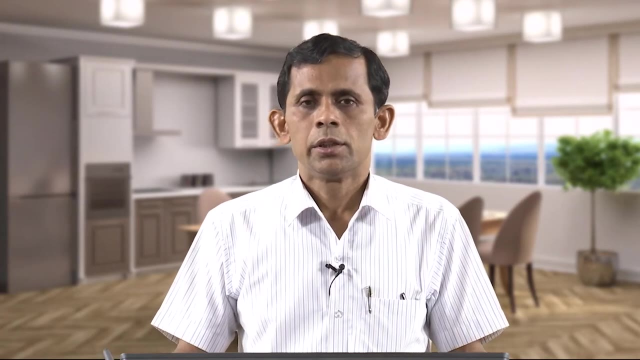 these we have VOC, CFC, Chlorofluorocarbon, and then NO2, Nitrogen Dioxide and Ozone. The sources of these pollutants we have already discussed. it can enter into the environment through natural sources as well as manmade sources, and some sources are also mentioned. 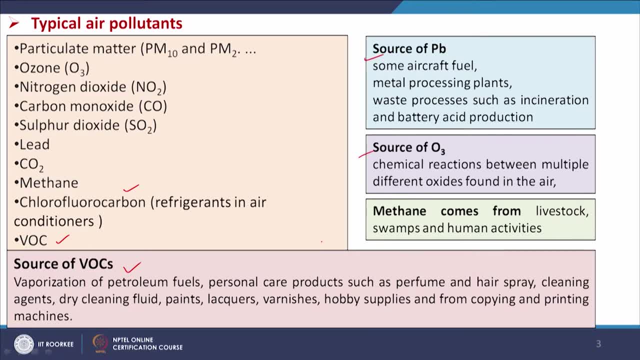 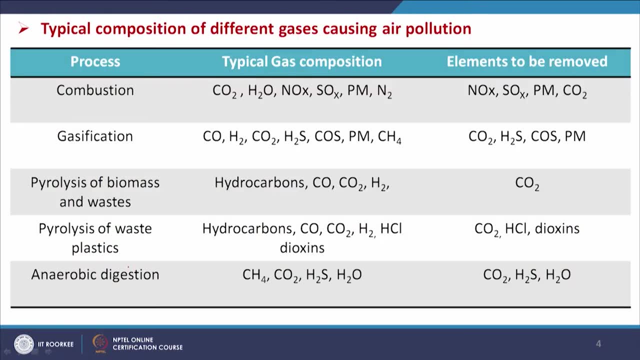 here, that is, source of lead, source of ozone and methane and volatile organic carbons. Now we will see different types of gases which are responsible for the generation of pollutants in the air. examples are, say, combustion gases. so when some fuel or carbonaceous material 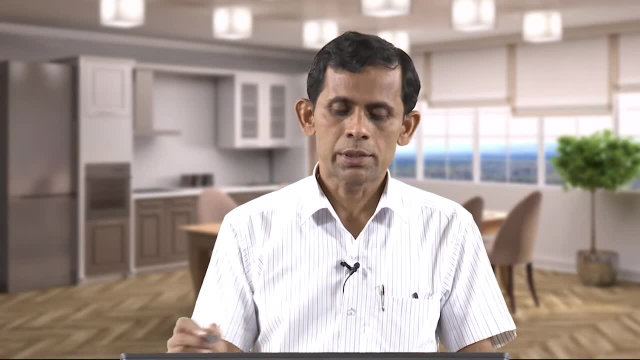 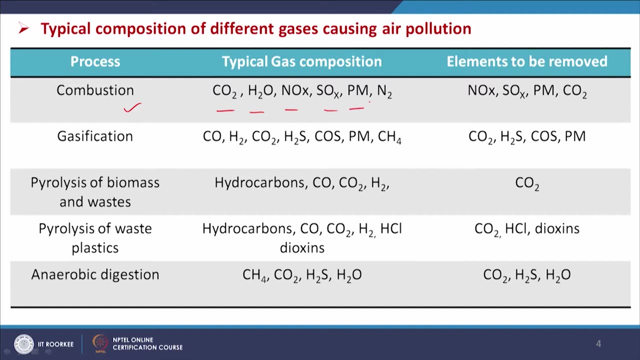 is combusted, then we get a flue gas which mainly contains carbon dioxide, NOx, SOx, H2O- that is in vapour, and particulate matter and nitrogen, and in this case we need to develop some methodology to remove these components like NOx, SOx, particulate matter and carbon. 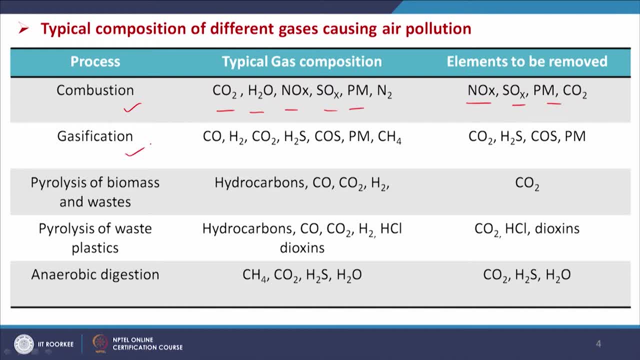 dioxide. So, similarly, through a gasification process, we can get different gas in the produced gas stream, like carbon monoxide, hydrogen, CO2, H2S, COS, PM and CH4. these are the major components and we need to remove these also: carbon dioxide, H2S, COS and PM, pyrolysis of biomass and 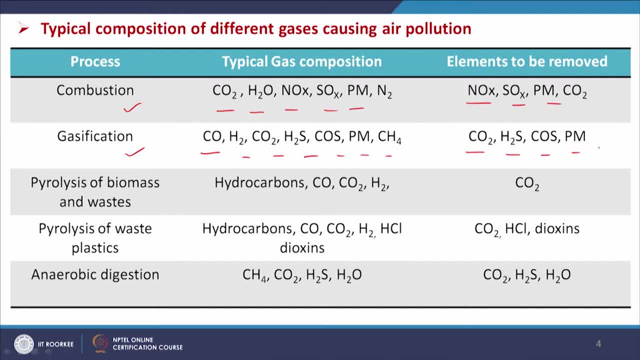 waste. through this route also, the gas comes out to the environment, which contains carbon monoxide, carbon dioxide, hydrogen, NOx, SOx, H2O. Now, at this point, these gas streams are very toxic, so we need to get such carbon dioxide. 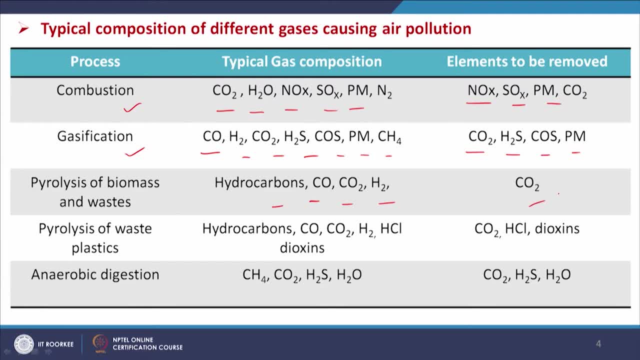 нашей Way and, of course, these gas streams are very toxic, so what we do? so, while we are here in the Mohawk area, I am going to explain you to understand what are many of them, which contains methane, carbon dioxide, H2S and H2O, that is, moisture or vapour and removal. 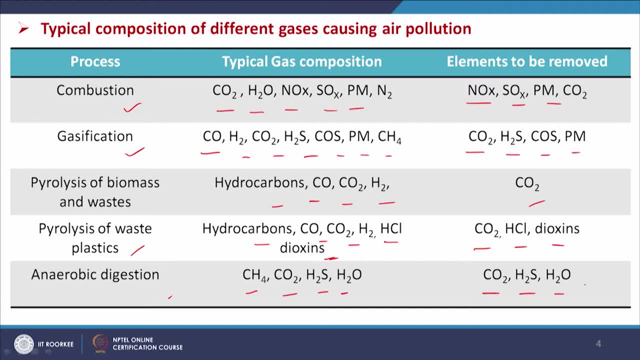 of CO2, H2S, H2O are very, very important, So these removal normally takes place in the premise where the gases are produced in industrial scale. Apart from that, so vehicular emissions, that is very difficult to control basically, and it contributes on the ambient. 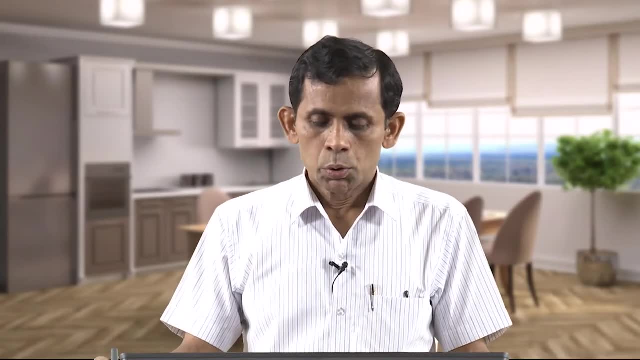 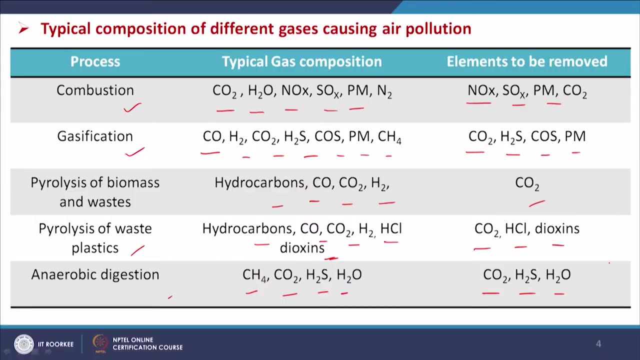 air quality. So to make the environment clean, we need to control the emission of these gas components. why needs get entry into the atmosphere? Here we have not mentioned regarding hydrocarbons. Hydrocarbons mostly is available in terms of unconverted emissions. 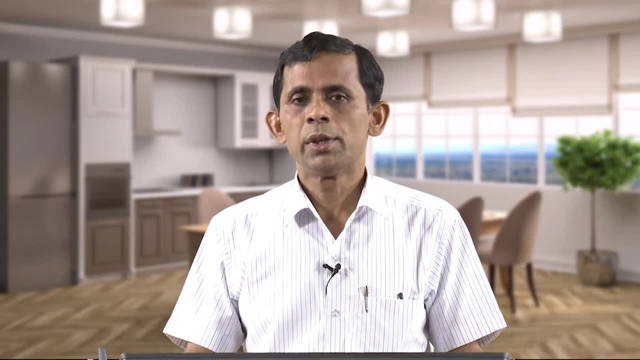 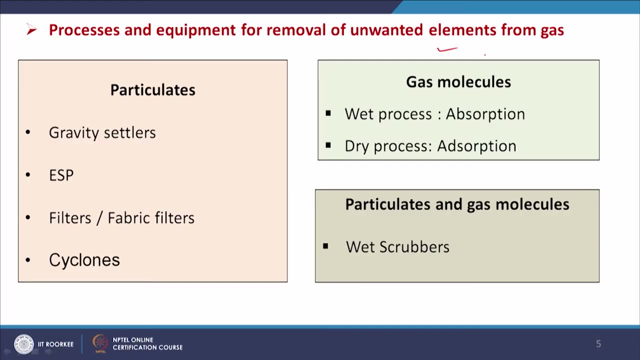 Hydrocarbons in terms of soots or it may be as volatile components, So volatile compounds, so those are also needed to be removed. Now we will see processes and equipment for removal of unwanted elements from gas. So in the gas, one is particulate matter and another 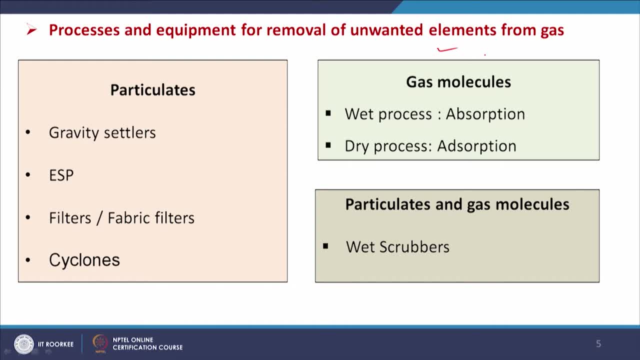 is other gas components we need to remove which are not desirable in the environment. So for the separation, For the separation of particles or the particulates, there are number of techniques and methods. we will be discussing those like, say, gravity settlers, then electrostatic precipitator and 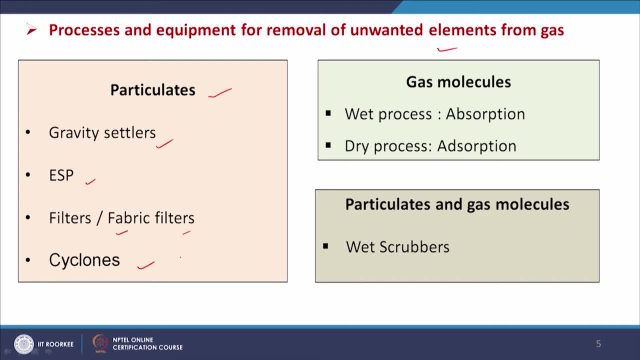 filters, that is, fabric filters- and cyclones. So these are the mostly used equipment or the processes which are used for the removal of particulates from the gas stream- So we will be discussing those- and for the removal of gas molecules, like, say, shocks, knocks. 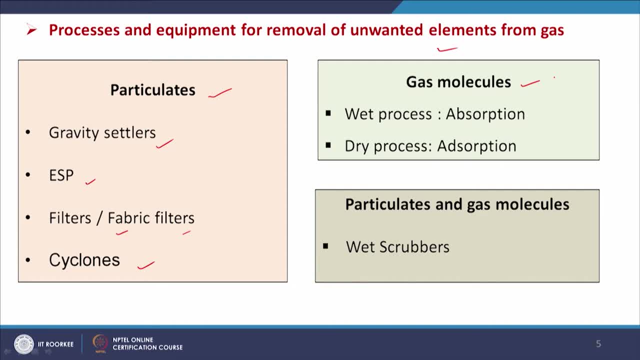 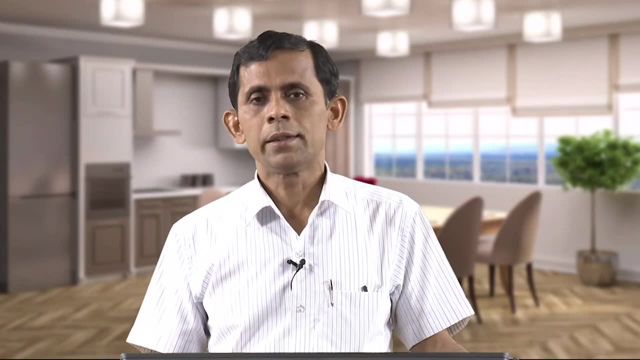 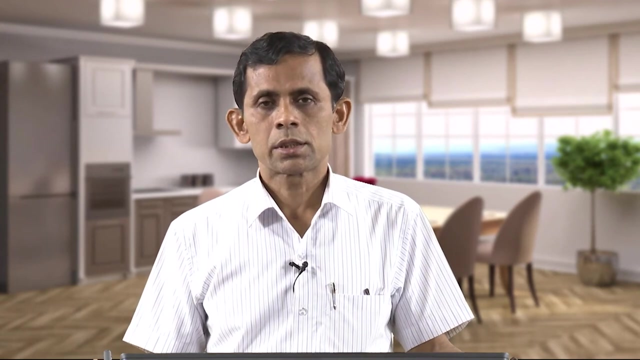 etcetera. There are two major methods. one is based on absorption, that is wet process, and another is dry process, which is based on adsorption. and there are some methods where both particulates and gas components can be removed, like say scrubbing, So wet scrubbers are also available. we will discuss all those processes and devices. 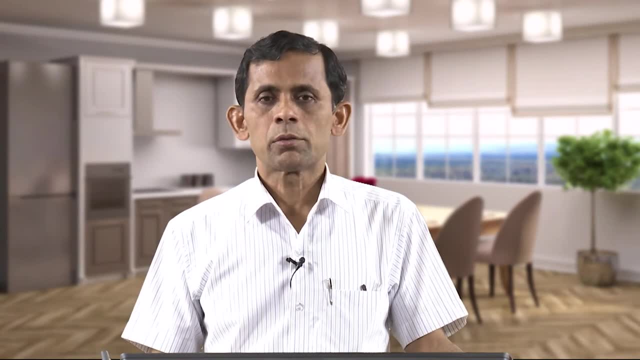 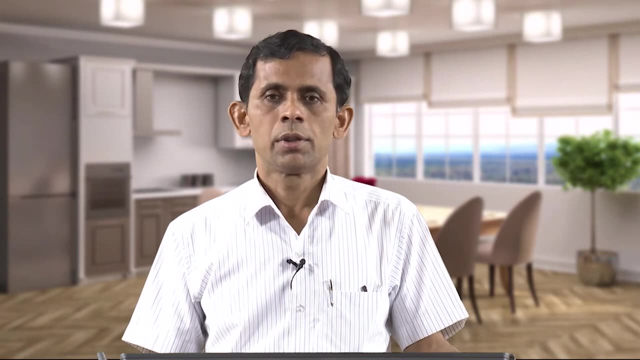 and we will learn how to remove the particulates and other gas components. Here we will also discuss sucubole. So with new device modernization it is important that we should components from the exit gas. and what are the mechanism of these equipment and the principle? 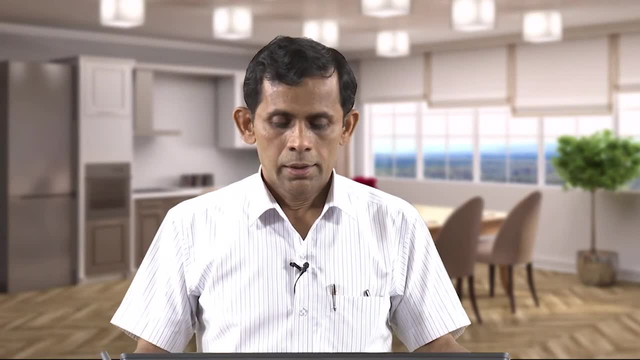 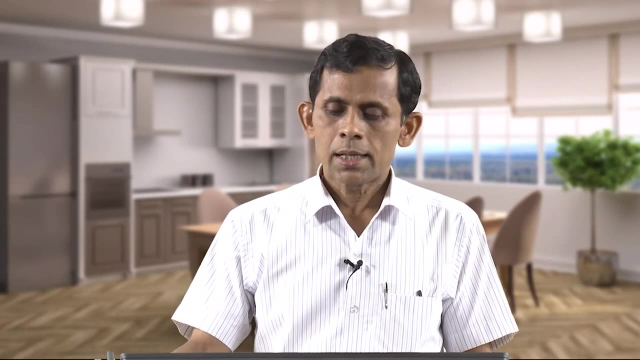 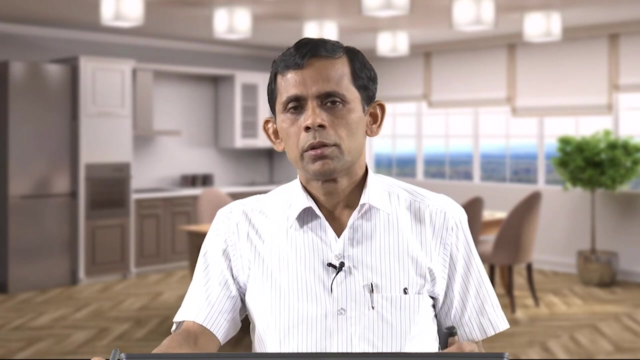 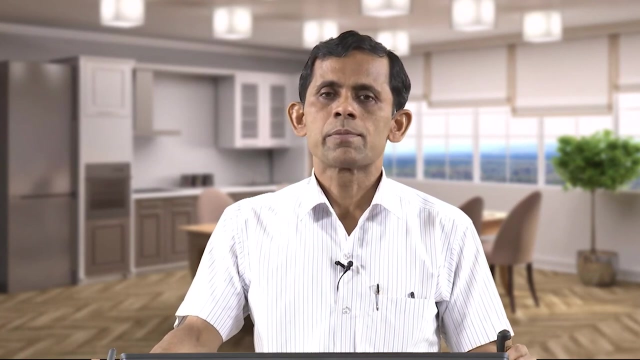 of working of these equipments, And in this part one we will be mainly focusing on the gravity settlers. So here this slide shows us a horizontal flow settling chamber. As you know, if we fall a ball or any particle from a height, so gradually its velocity will 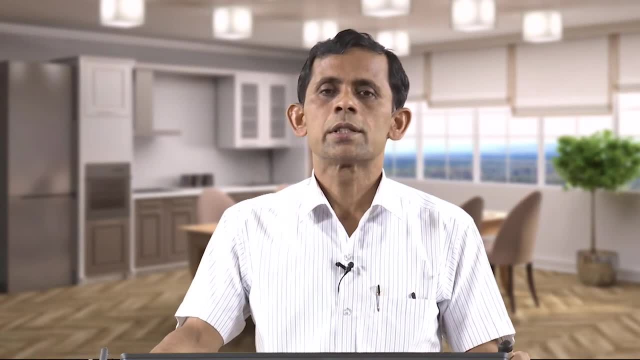 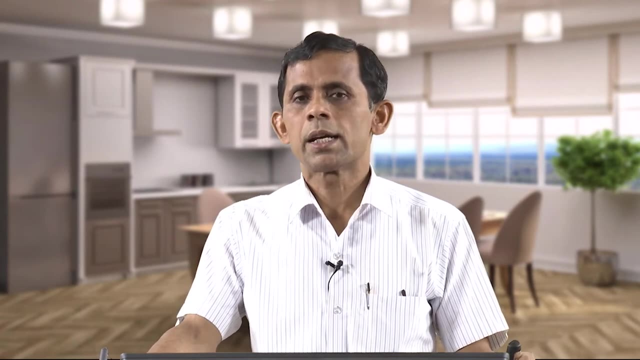 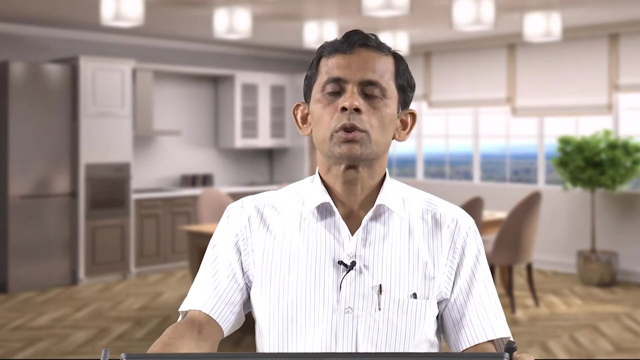 increase. Initially the velocity is 0, then gradually its velocity will increase and it will attain a maximum velocity that will be stable thereafter. that is called terminal settling velocity. So this terminal settling velocity- bigger the particle size, more the terminal settling velocity. So to achieve this we will have to use a 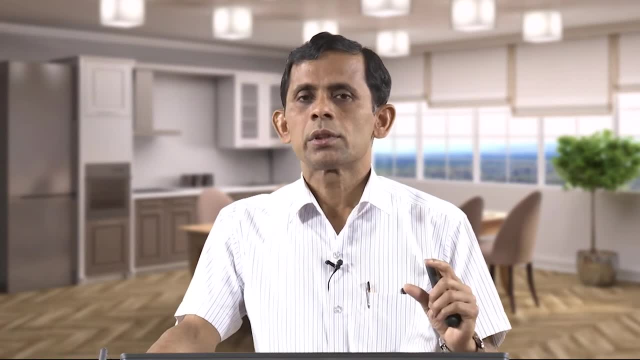 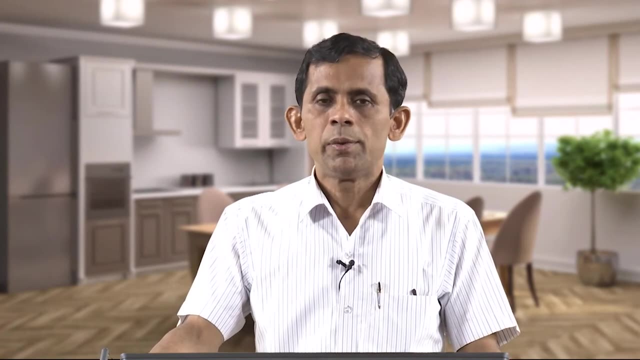 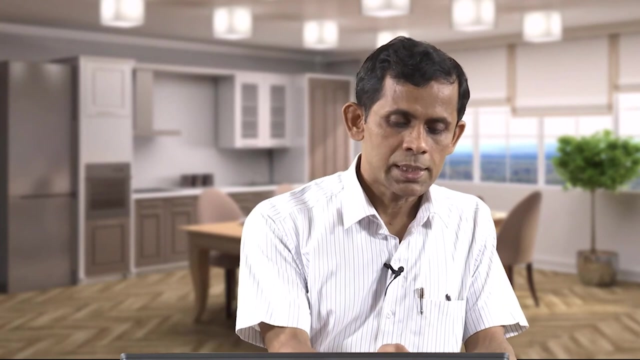 principle: to travel a certain distance, the more the terminal settling velocity, lesser the time required. So the same principle will be applicable for the separation of the particles in the gravity settlers. So this figure, if we see so, here is the gas in. so 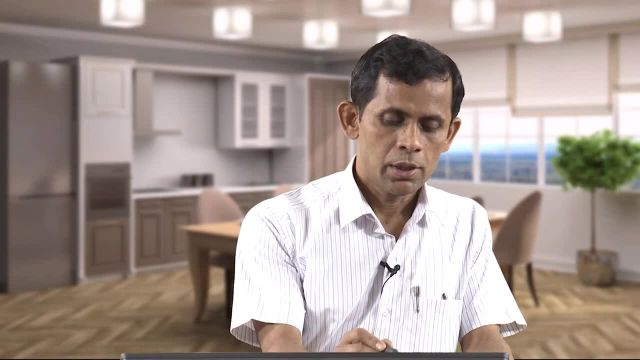 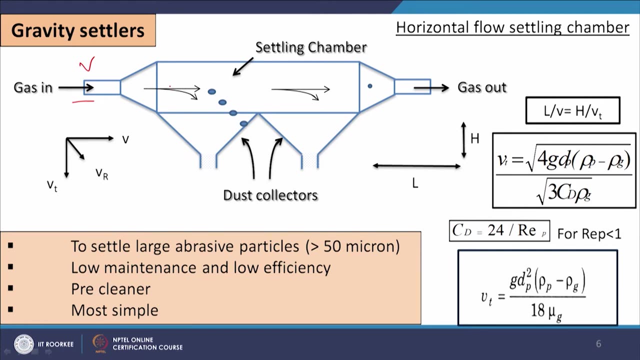 inlet gas is coming here, So it will be having some velocity, so that velocity is equal to say v. So this velocity gas is coming, so if particles are present in it, so that particles will also be having the velocity v, and here the gravity is also working on the particle. 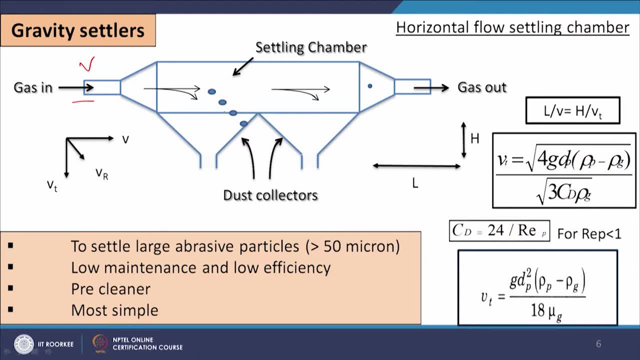 So the particle is under the action of multiple forces, so one trajectory you will get through which this particle will move. So now it is having a horizontal velocity v and vertical velocity vt, that is terminal settling velocity. So this is our resultant velocity. Now, if 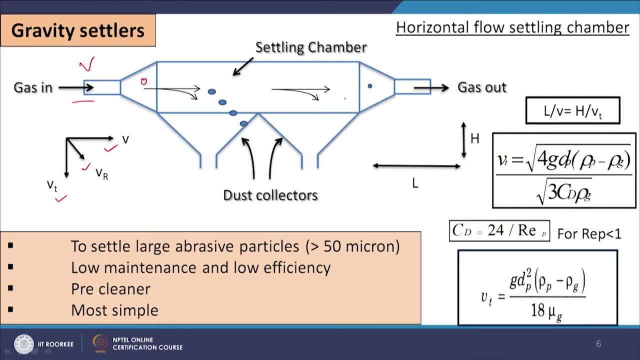 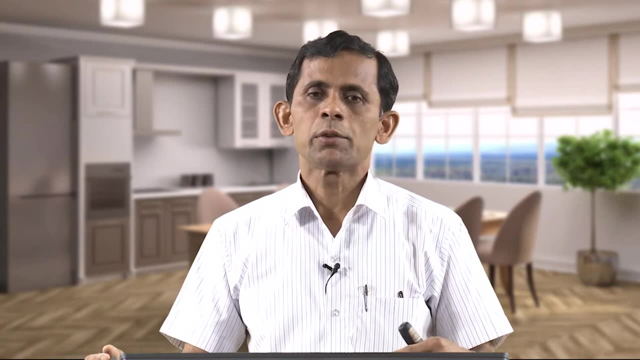 If you see, one particle is here so I want to get it separated. so the basic principles of separation of any particles while it is in motion, just if we can put something in its path and then its flow will be arrested and the velocity in that particular direction. 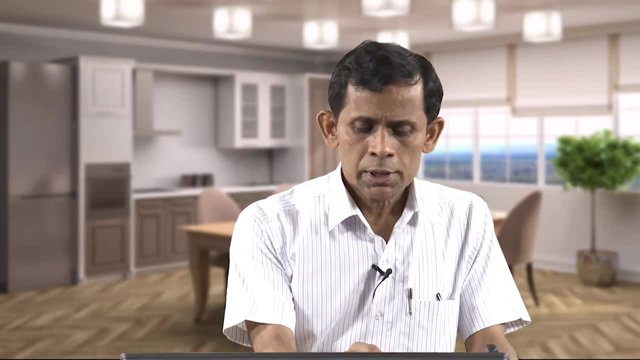 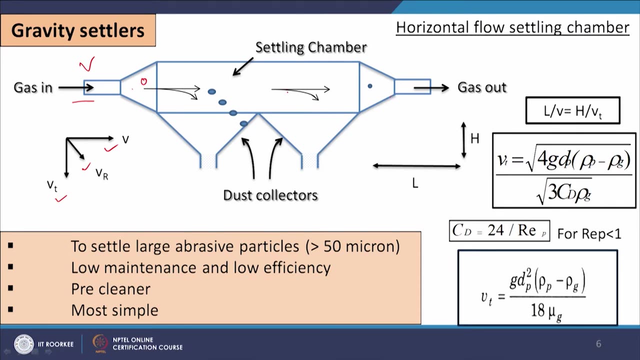 will be 0 and the particle will fall. So if this particle we want to settle here, certainly the time required to travel from this point to this point the inlet to outlet within this time the particle must travel the vertical distance which is the as per the dimensions of this settling chamber. 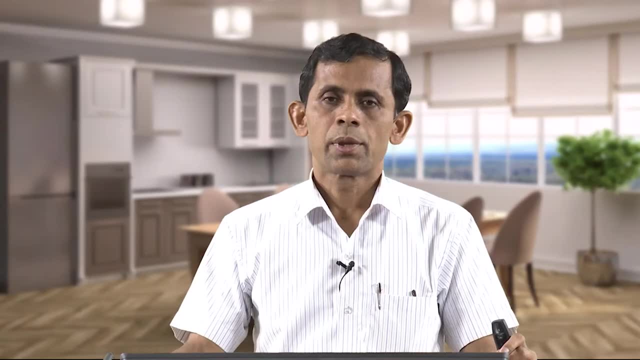 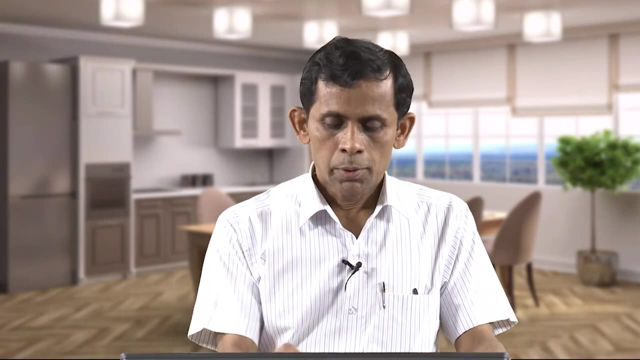 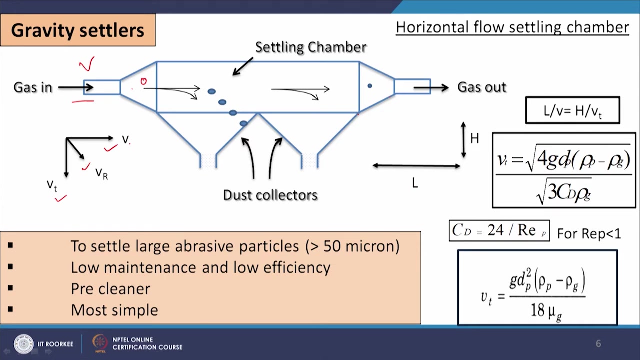 So this is the basic requirement or the design principle for this settling chamber. So if we consider the length is l and height is h, so in this case l by v, v is the horizontal velocity, So l by v is the horizontal velocity, So l by v is the time required to travel from inlet to outlet by the particle, and h by v. 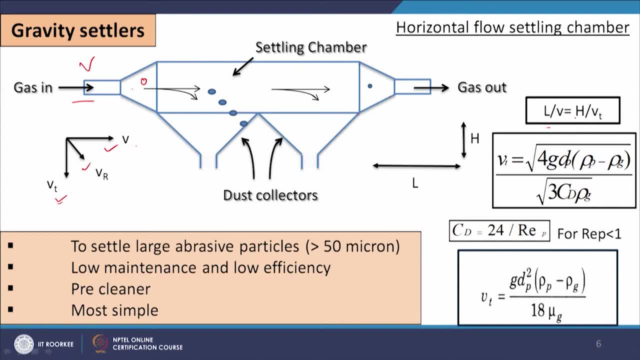 t, where v t is the terminal settling velocity, that is the time required to travel the particles from the top to the bottom of this chamber. So this time requirement should be equal. So this is the critical condition for the separation. So l by v equal to h by v t. 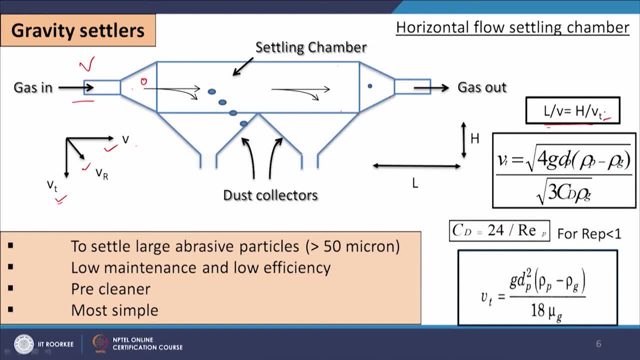 Now this v t is equal to what v t is terminal settling velocity, and terminal settling velocity will depend upon the particle size, the viscosity of the fluid, the density of the particle, etcetera, and what is the g value, that is, the gravitational acceleration. 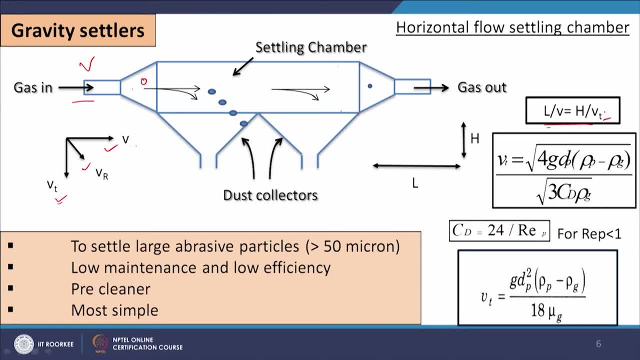 So those values will be influencing the value of v t and v t is equal to root of 4g d p, rho p minus rho g, divided by root over 3 c d rho g. So these expressions we will discuss. So this expression we will discuss, and from this is coming: 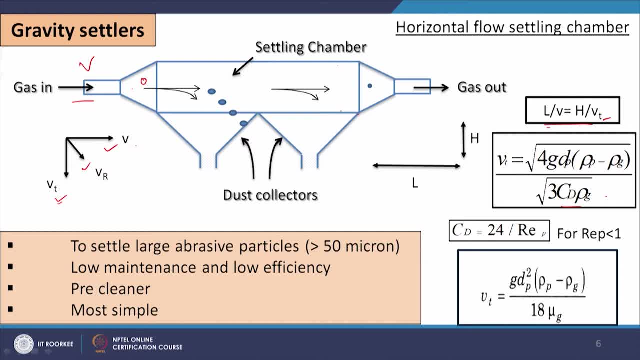 is coming by, the force balances on it and this C- D is nothing but the drag coefficient. So this drag coefficient will be depending on the velocity of the gas stream. So the velocity is higher, that is your. it will be in turbulent. but velocity is less we will. 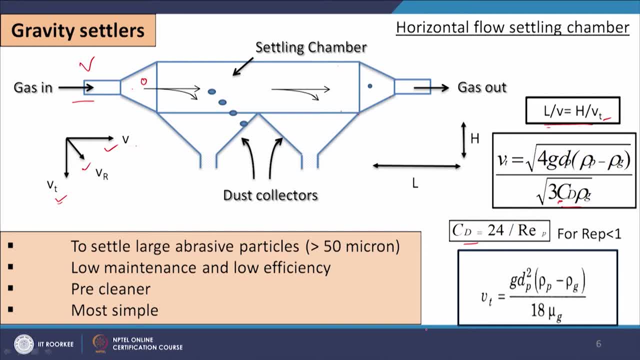 be getting. this is in laminar flow. So up to certain Reynolds number we will be getting laminar flow and in that case, and the Reynolds number is less that, we will be getting the laminar flow and in that case C D is equal to 24 by R ep. R ep is nothing but the particle. 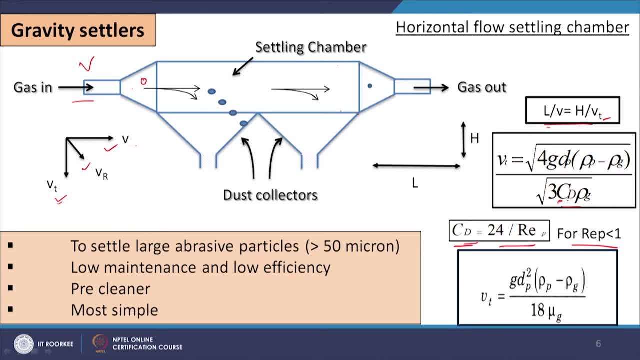 Reynolds number. So this C D value we can. we can replace it by 24, by R ep. so V? t will be converted to g d p square rho p minus rho g by 18 mu g. So this expression is the expression. 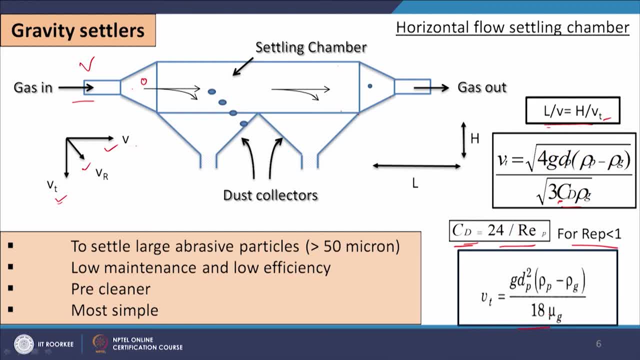 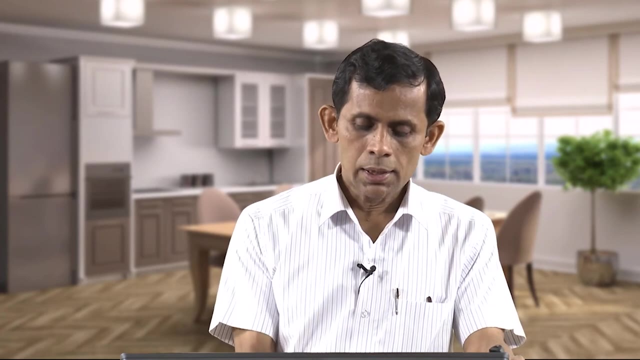 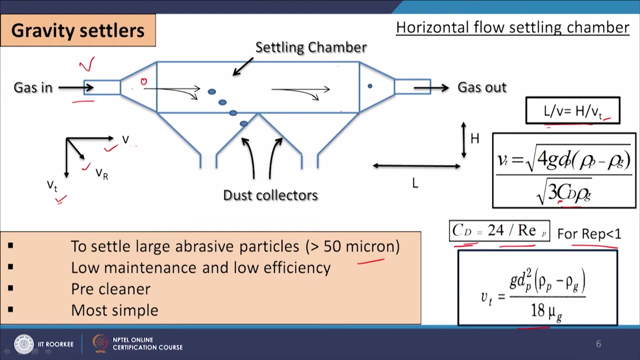 for the terminal settling velocity of a particle which is falling in laminar zone. the flow of the particle is not that high, so that the Reynolds number be less. and this equipment, the gravity settlers, are very simple and it is not costly and to settle large abrasive particles like, say, greater than 50 micron. this device is workable and 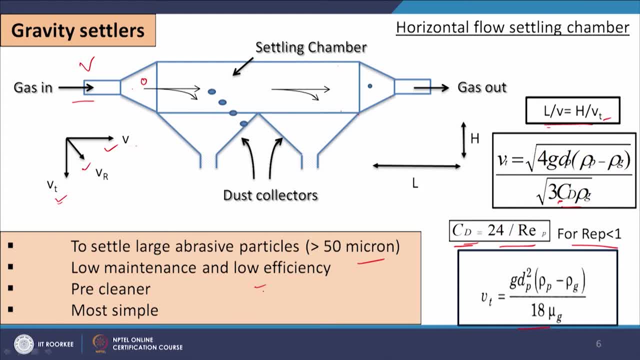 it has low maintenance and low efficiency as well, and it is also considered as pre cleaner. So for the separation of very fine particles it may not be that good device, but for the separation of relatively larger particle this can be a good option, and this is a very simple 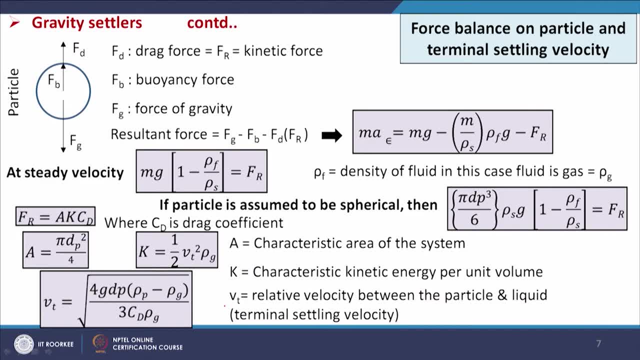 method. Now we will see how the Vt expression we are getting. So let us see: this is the particle which is falling. So there is one force, that is Fg, that is gravitational force, which is working in downwards direction, So upward directions. one force is working, that is Fb, that is buoyancy force. as you know, when a solid particle falls, 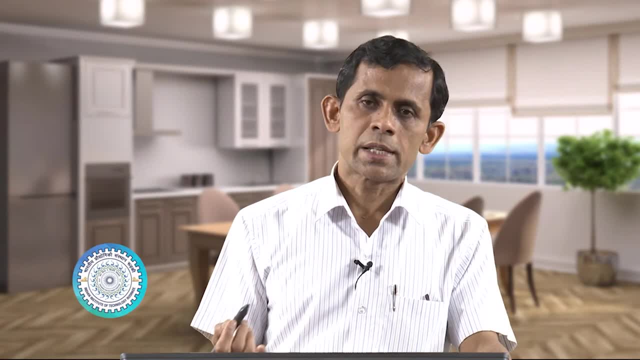 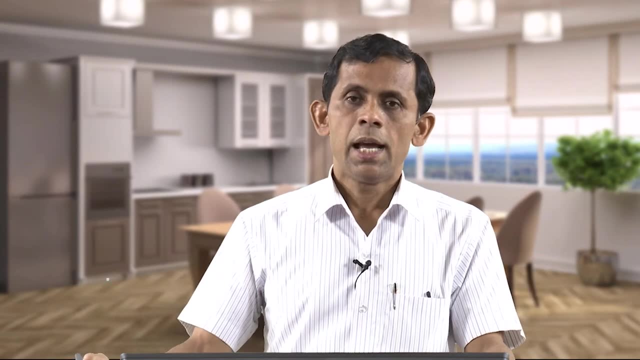 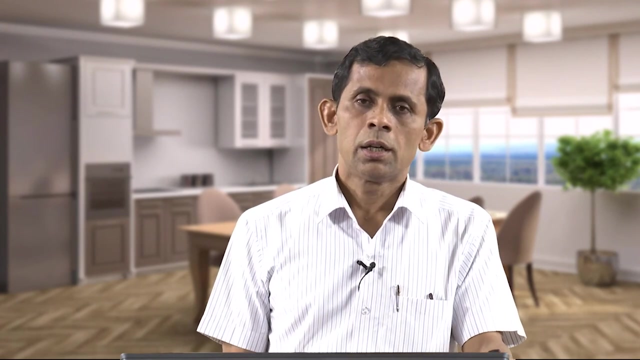 then in a fluid. then fluid is replaced, same volume of fluid is replaced and it gives a force to the particle in opposite direction. so that is buoyancy force. and another force we will be seeing here, that is drag force. So this drag force is also working on this particle when it is falling in the air show. 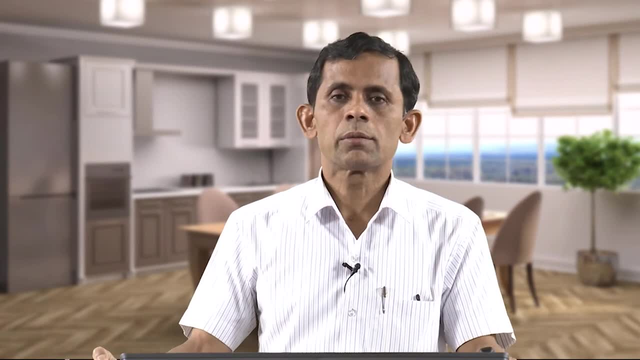 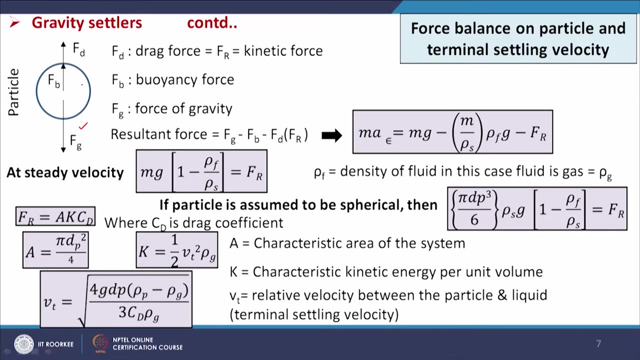 that drag force will also work in the same directions of the buoyancy force opposite to the gravitational force. So if we think about the force acting on this particle and we consider the force balance, then we can say that the resultant force on this particle is equal to the force due to gravity, minus force due to buoyancy, minus force due to gravity. 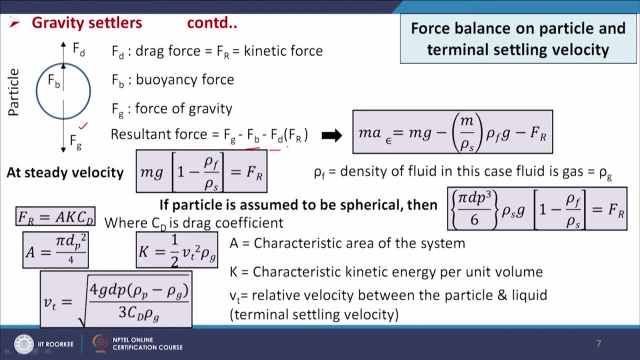 drag. So these are Fg minus Fb minus Fd. So this drag force is basically mentioned as kinetic energy force. So in many books it is written as Fr. that is related to the kinetic energy of unit volume of the fluid. So this is the expression for the resultant force on this particle. 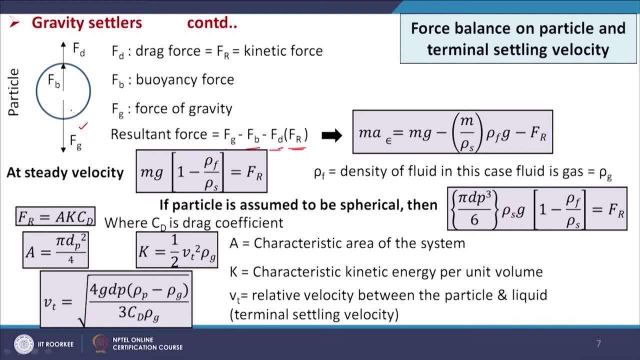 Now when it will be moving with terminal settling velocity. so there will be no resultant force, So that it will be moving in the constant velocity that is terminal settling velocity. So in this case we will be getting resultant force equal to 0.. So now let us express this resultant force. 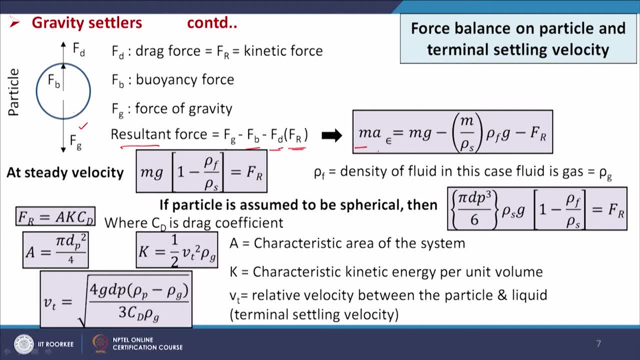 So M is the mass of the particle and Ae is the resultant acceleration. So M into Ae, that is the resultant force. So that is equal to M into g. that is gravitational force minus minus buoyancy force. that is m by rho s into rho, f into g and this is our Fr. so Fr is: 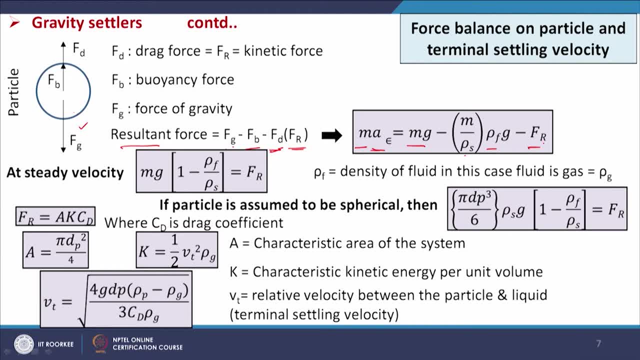 the drag force. so drag force, as I mentioned, it is related to the kinetic energy of unit volume of the system, unit kinetic energy per unit volume. so Fr is equal to A into Kd, into Cd. so A is the cross sectional area and K is the characteristic kinetic energy. 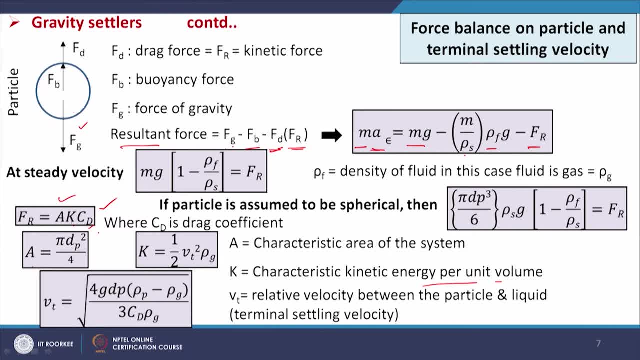 per unit volume and Cd is nothing but the drag coefficient. so K which we are talking about, that is half into Vt square, into rho g. so what is half mv square? so if I take one volume, unit, volume of the fluid, so V into 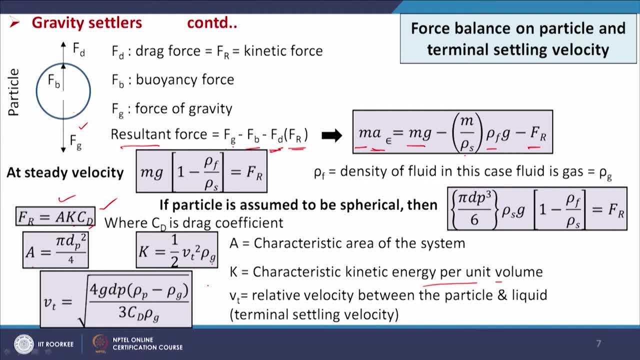 rho g, so that is equal to mass of the fluid, and then half mv square, that is kinetic energy of the fluid. so this is the expression of K and the expression of A. A is nothing, say a particle is falling from this. so we will be taking the cross sectional area here. so 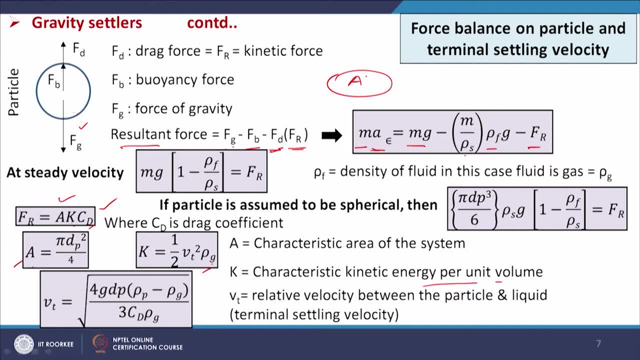 the cross. this cross sectional area is A, so then this A will be pi r square, so pi dp square by 4, so this is our A, the K expression we have described. so if we put the value of A and K in this Fr and also put the values of this Fr here in this expression and put 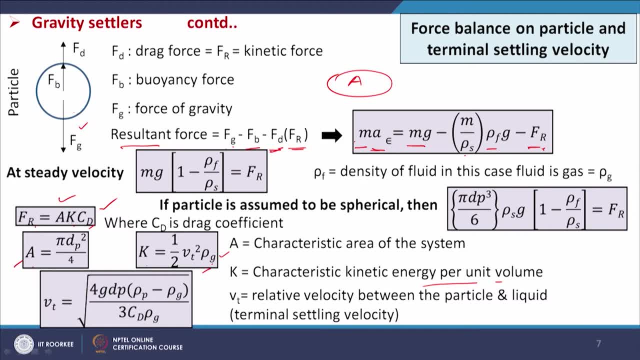 ma equal to 0, then we will be getting the value of Vt. say, in this case, what is Fr is equal to mg minus m by rho s into rho f, into g. so we will take the common, that is, mg so 1 minus rho f by rho s, and this m term is taking common so m, if we are interested. 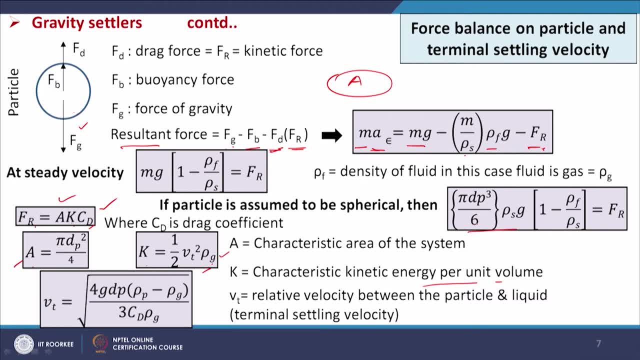 to convert this m in terms of volume, because you know we cannot measure the weight, we do not need to measure the mass. but dp is known to us so we can get the volume. so accordingly, mass can be converted to this volume. so pi dp cube by 6 into rho s, into. 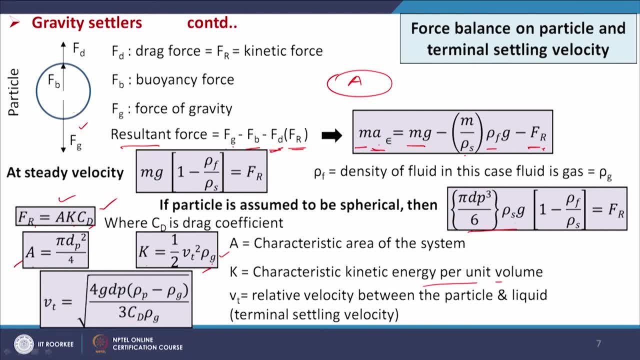 g, that will be the m if we consider it, the particle, as a spherical particle. so when we will be considering the particle as a spherical particle, so this expression will be like this: So here Fr value we will be putting like Ak, cd and A value is given, here K value is 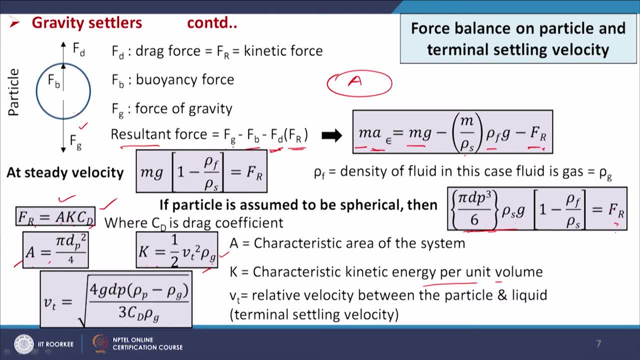 given here. we will put this expression here. so by rearranging we will be getting. the value of Vt is equal to root over 4 g dp into rho p minus rho g, divided by 3 cd into rho g. so Vt is the terminal velocity between the particle and liquid and the fluid in this. 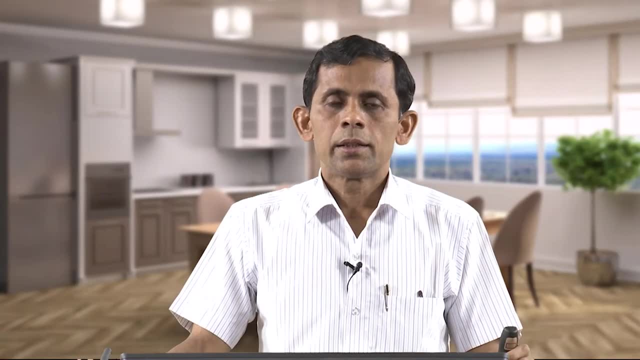 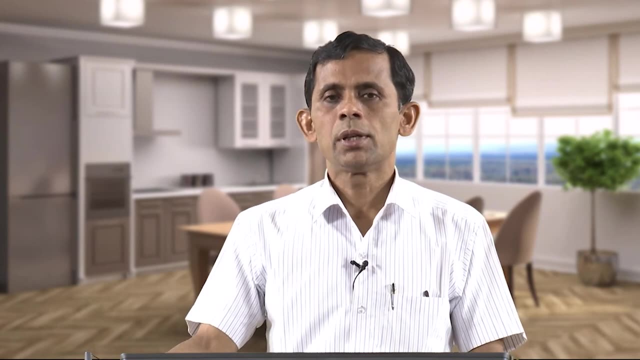 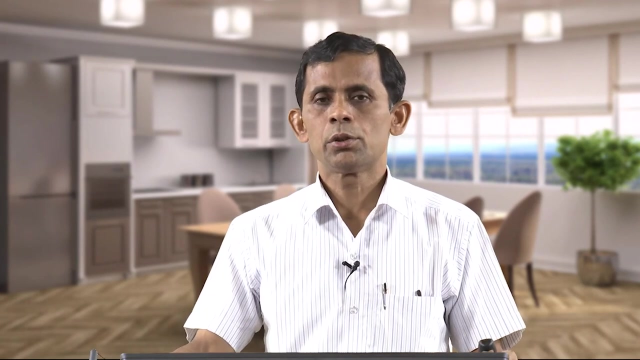 case that is air. Now we are able to understand now How The particle will be separated in the gravity settler and how the Vt value can be calculated Now, how the collection efficiency can be calculated, because you know, the more the particle size 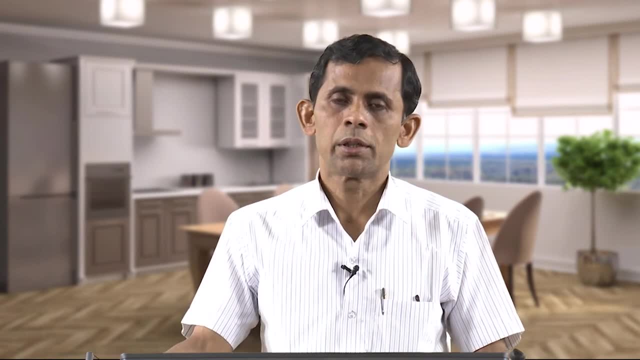 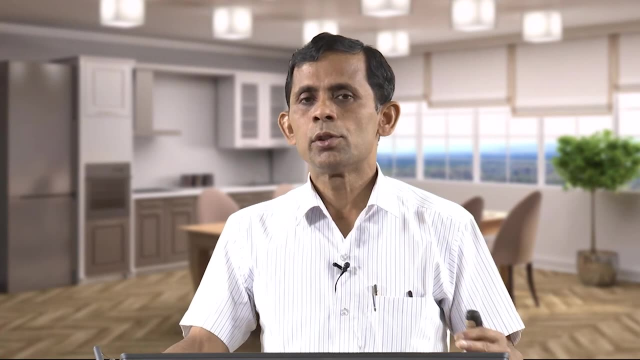 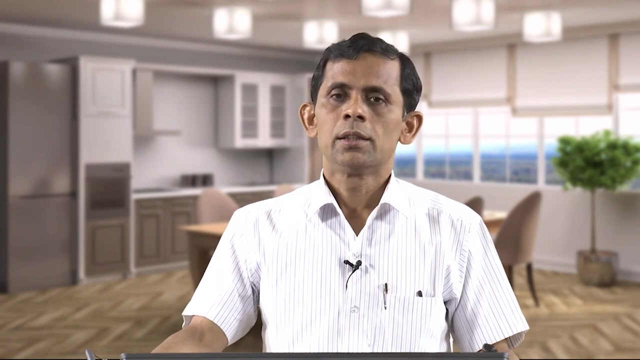 more will be the terminal settling velocity, less will be the time requirement, so the time required to travel from inlet to outlet. within this time all particle size will not be equally settled. so bigger the particle, more easily settled. lighter the particle, it will be lesser settled. so we can get one cumulative analysis on the, if we say x axis. 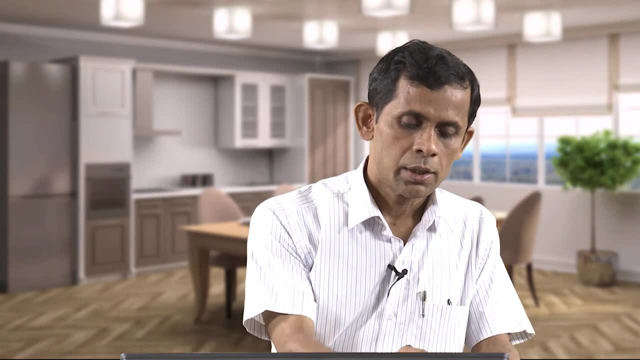 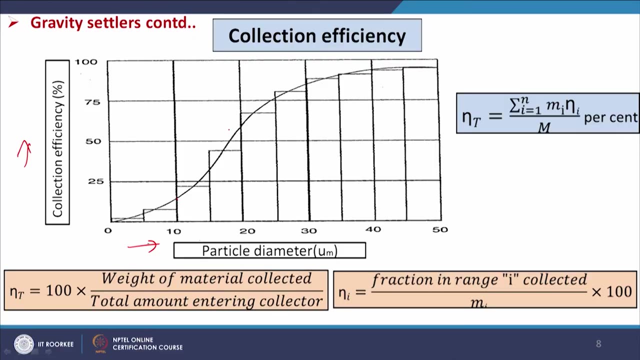 if we plot the particle diameter and y axis, if we write the collection efficiency, we will see that when the particle diameter is less the collection efficiency will be less, but gradually it will increase cumulatively. we can get at the maximum collection efficiency when we will be considering the particle size in the higher range. 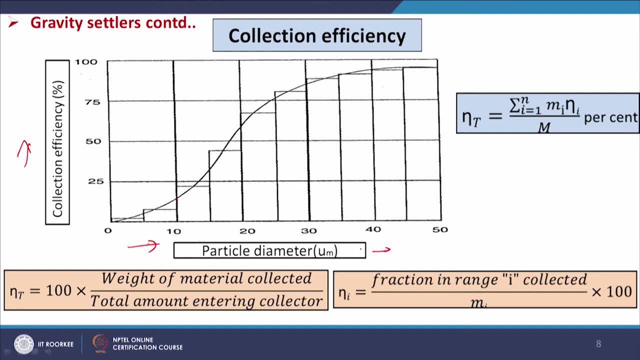 So that way it is physical. So now, mathematically, if you want to express, then you can write that eta t is equal to 100 into weight of material collected, by total amount entering in the collector. and this eta t is equal to sum of i equal to 1 to m and m i n, i by m. 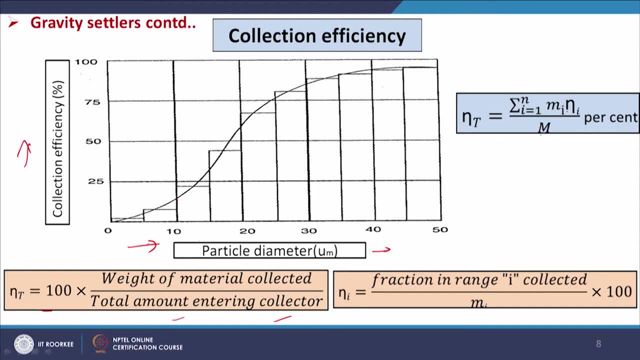 So sum of i equal to 1 to n m i, eta i by m. so eta i is nothing but the fraction in range i collected by m i is the mass, total mass of that fraction collected into 100.. So that way we can calculate the collection efficiency by using this formula. 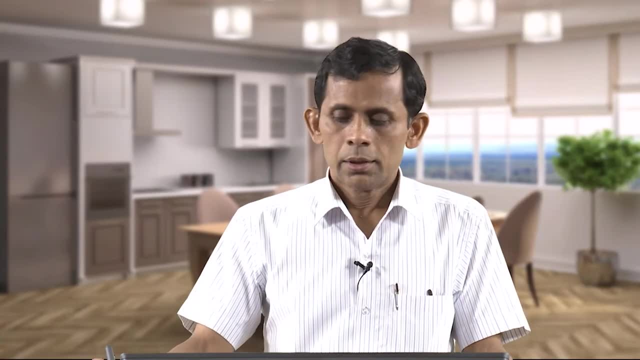 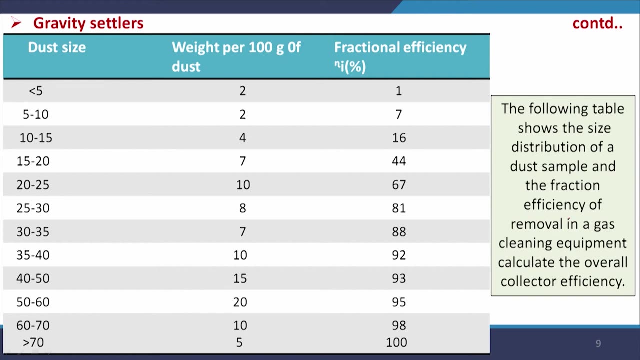 Now we will see one numerical problem. so the following table shows the size, distribution of a dust sample and the fraction efficiency of removal in a gas cleaning equipment. calculate the overall collector efficiency. So this table is given. So dust size less than 5, and then weight per 100 gram of dust equal to 2,, 2 gram and 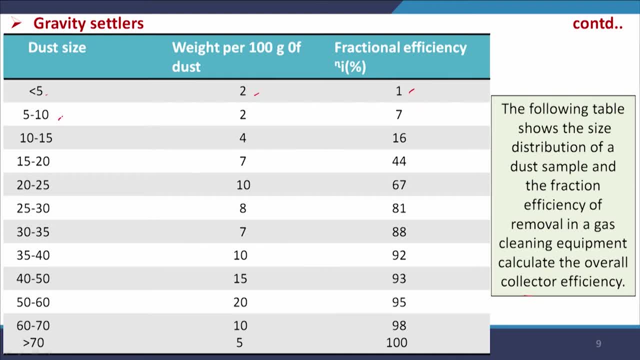 then fractional efficiency is given, that is 1.. Similarly, for 5 to 10, it is 2 and it is 7, and 10 to 15, it is 4 and 16, so 15 to 20, 7 and 44.. 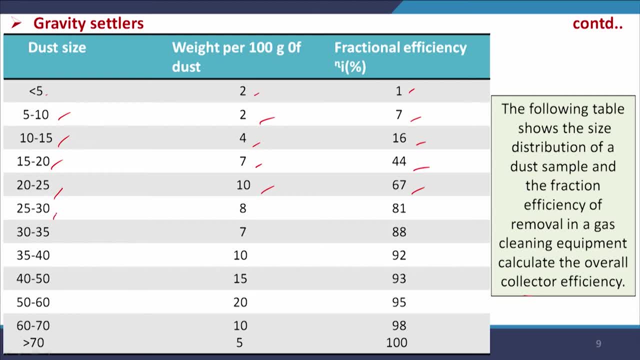 So 20 to 25, 10 and 67 and 25 to 30, 8 and 81 and 30 to 35, 7 and 88 and 35 to 40, 10 and 40 to 50, 15 and 93 and 50 to 60, that is, 20 and 95 and 60 to 70, 10 and 98 and greater. 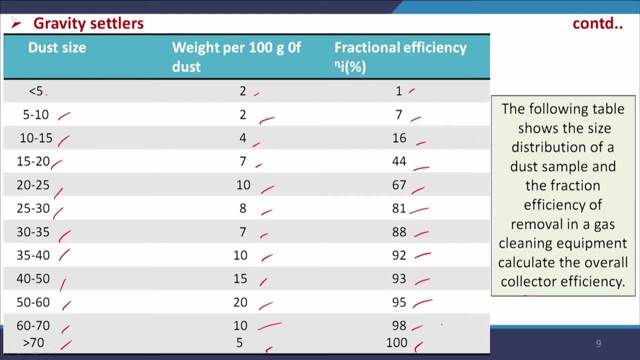 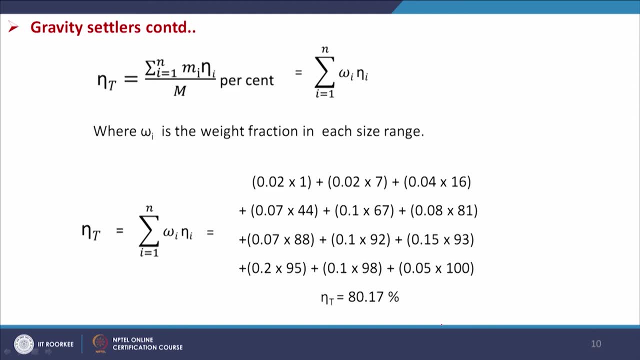 than 75 and 100.. So we are getting. this is the data given to us. we need to calculate the collection efficiency. So how we will do it, we have the formula eta: t is equal to sum of i, equal to 1 to n. 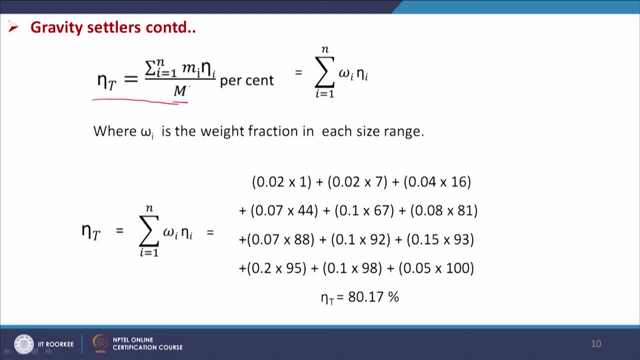 sum of m i eta. i by m, So m, i by m. So this is nothing. This is nothing by wi. so wi is the weight fractions in each size range. So mass fraction and weight fraction, both are same. So in this case, as per our statement, you see, if we apply this formula, sum of i equal 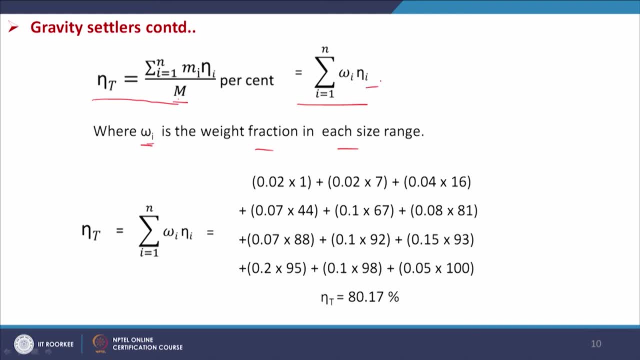 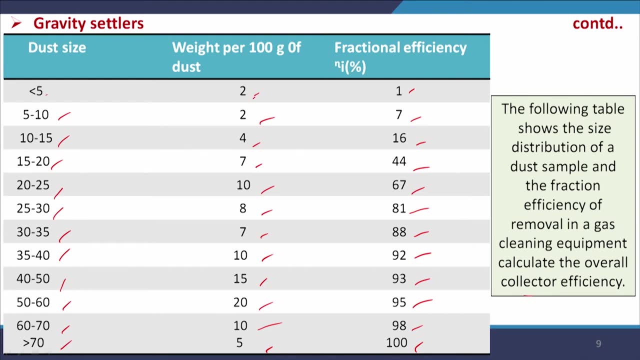 to 1 to n wi eta i. so we have to find out the wi value. wi is nothing but m i by m. So in the first case 2 gram that is m i and total is 100 gram. So 2 by 100.. 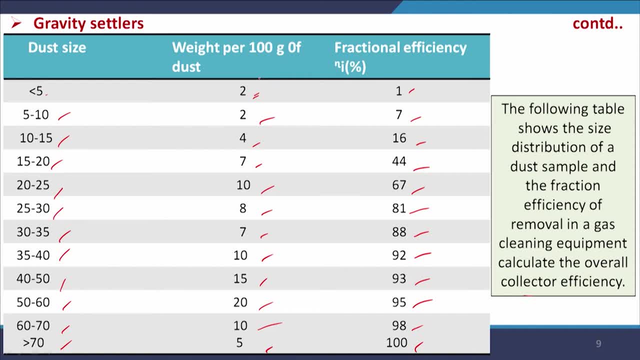 So this is our m i, small m i. it is equal to 2 by 100 for the first case and for the second case, also 2 by 100. for the fourth case, 4 by 100.. So, and efficiency is 1,, 7,, 16 respectively. 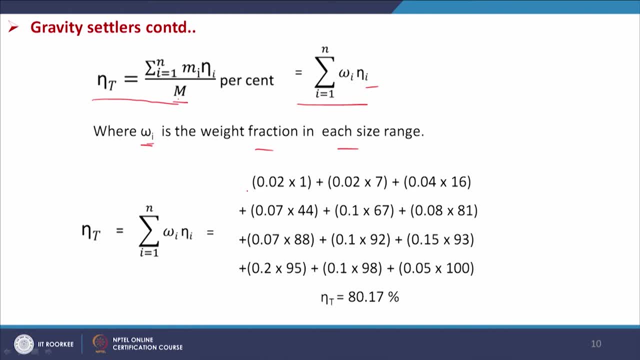 So we will be using this formula 0.02 into 1 for the first case. second case: 0.02 m i by m 0.02 into 7, that is equal to eta i. For the third case, it is 0.04 into 16 eta i. 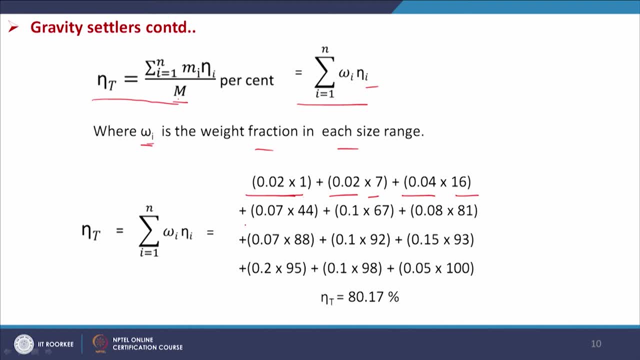 So 2 by 100 say we get What is the weight. So similarly, for other cases also, we will be getting 0.07 into 44 plus 0.1 into 67, plus 0.08 into 81, as per the data given in the previous table. So plus 0.07 into 88 plus. 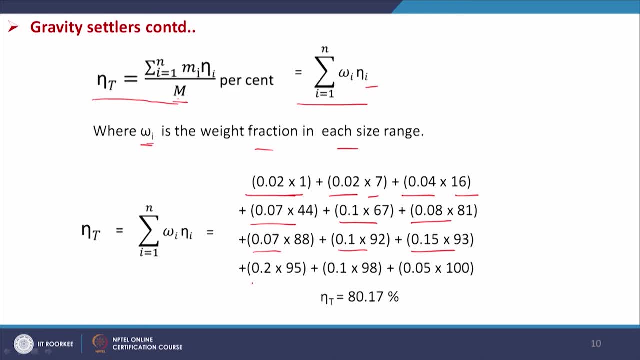 0.1 into 92, plus 0.15 into 93, plus 0.2 into 95, plus 0.1 into 98, plus 0.05 into 100. So it is coming as 80.17 percent. So now we are able to calculate the collection efficiency. 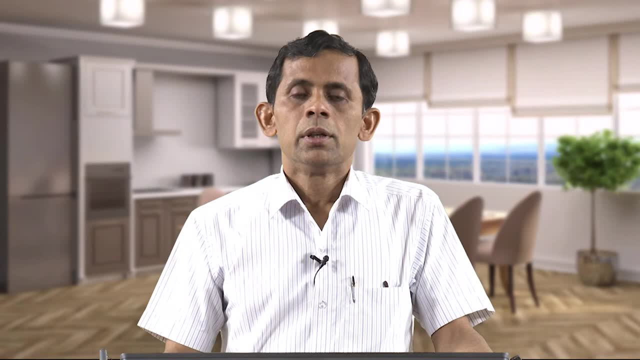 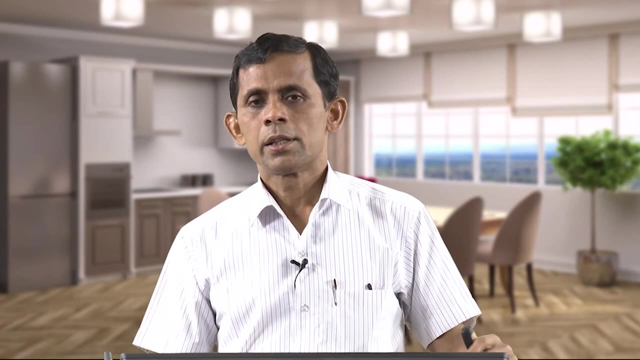 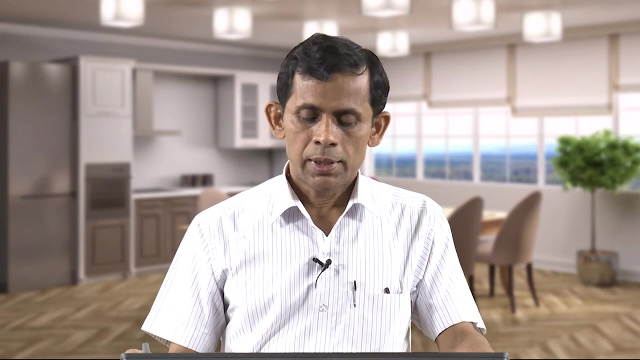 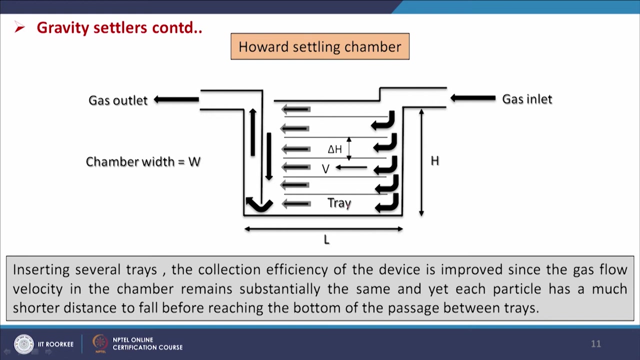 as 80.17 percent. Now. in practice you know, if we can reduce the height for the separation, then more separation is possible. So if we have a like this figure, if this is our height, in this height if we place some horizontal trays, So in between entire tray distance, 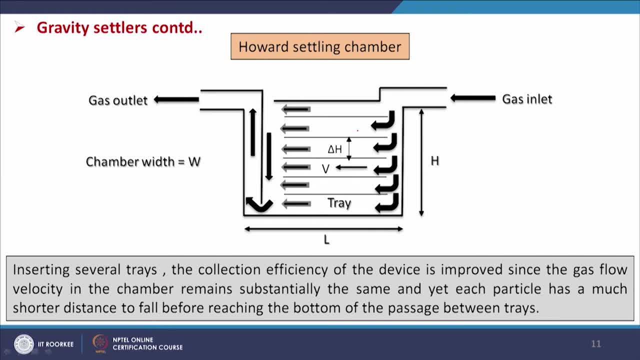 will be reduced, so air will pass through it. so particle need to travel vertically from this point to this point when, in the same time, when it is moving from inlet to outlet, but we do not put any internal shear or any plates inside, so then the particle has to remove from this. 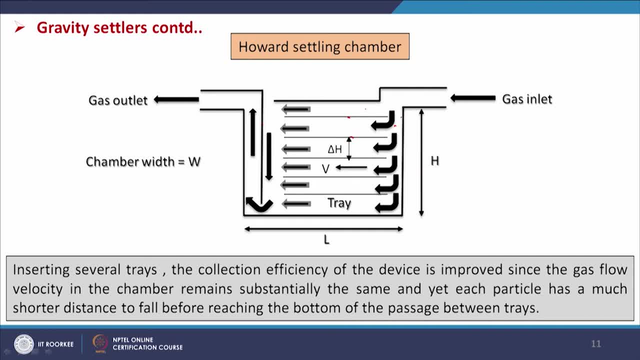 to this the complete edge height during the time when it will travel the length. okay, So by inserting these plates we are provide, we are reducing the vertical length for travel by the particles, so more separation is possible. So inserting several trays, the collection efficiency of the device is improved, since 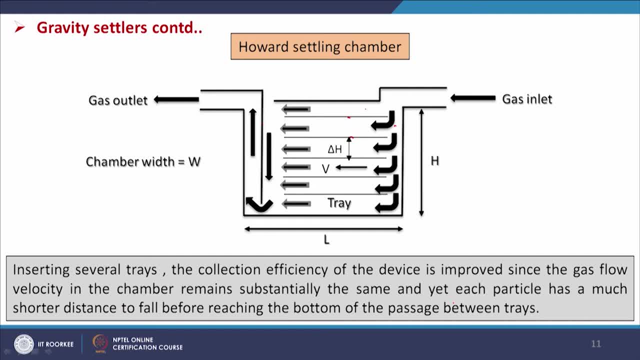 the gas flow velocity in the chamber remains substantially the same, and yet each particle has a much shorter distance to fall before reaching the bottom of the passage between trays. So, in this case, what will be the, The mathematical expression that we are going to discuss? okay, so for a settling chamber. 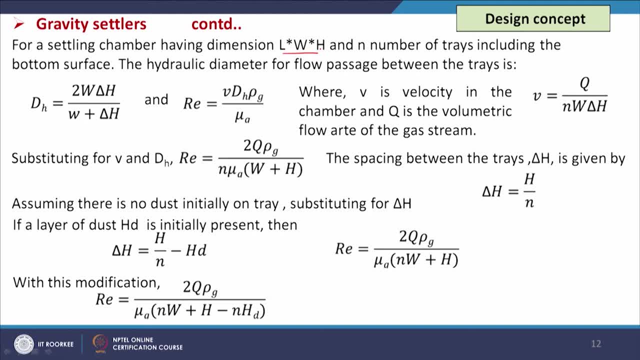 having dimension LWH, so L is the length, so W is the width. say WL and this is our height. so in that case, and n number of trays, including the bottom surface, the hydraulic diameter for flow passage between the trays is. then, if I want to calculate the hydraulic 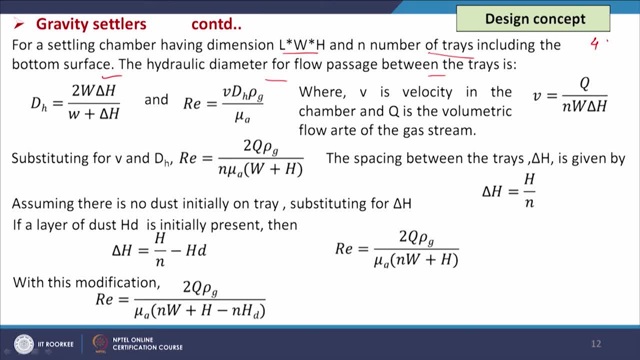 diameter, that is 4 into area. Okay, Okay, Okay. So 4 into area divided by perimeter. so 4 into area by perimeter. so in this case, say this is our W and del H is this side. so water is air is flowing from this direction. so 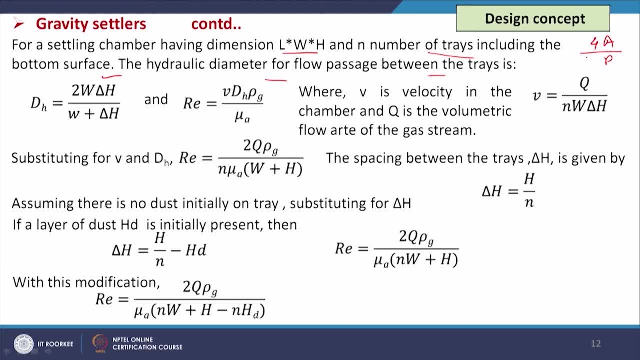 this will be our surface area, so W into del H, so W into del H is your A, so 4 into W into del H, divided by your perimeter, so perimeter, this is our 2 into W plus del H, so 4 will. 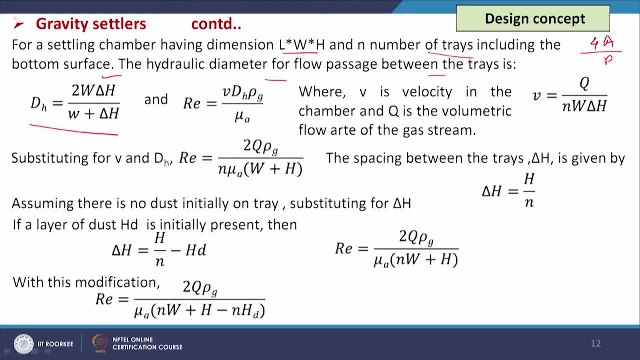 cut So that D H will be 2WH by W plus del H and we will be getting the Reynolds number. we know that rho D V by mu, so rho D V by mu will be putting here, so D will be this characteristic. 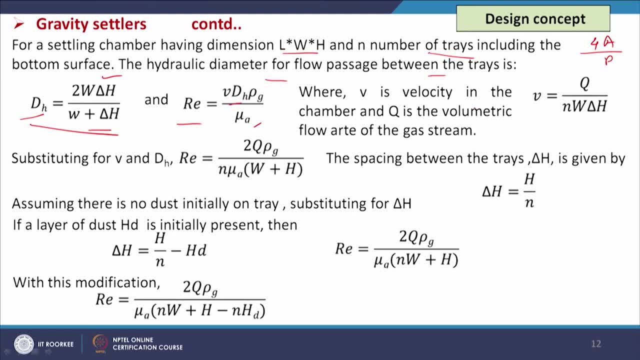 diameter, that is D, H and V is the velocity in the chamber. so this is our Re. So now, if we want to get the value of V in terms of the known dimension, that is, that is, W and del H, then we can calculate: V is equal to Q divided by N, into W, into del H. 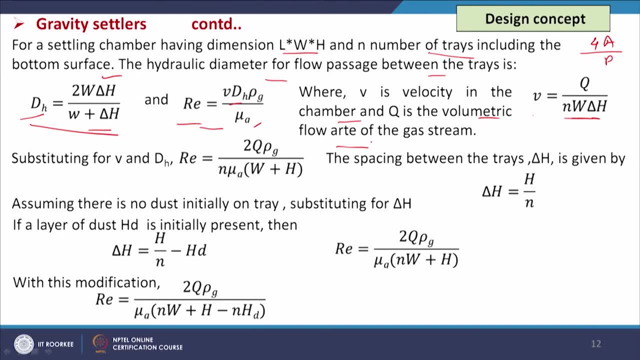 when Q is the volumetric flow rate of the gas stream. so gas is passing through this direction. so Q divided by cross sectional area, which we are getting W into del, H into N, N is the number of that channel, so that will into V, that will be the Q. so V is equal to Q. 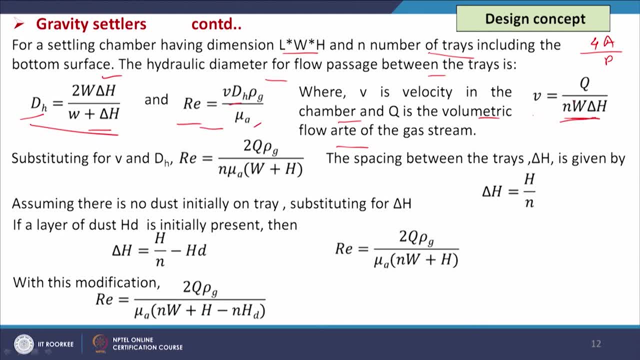 by N W into del H. So if we put this value V here, so Re will be converting to 2Q rho G divided by N, into mu G, into W plus H. so this expressions we are getting for Re now, when we do not have. 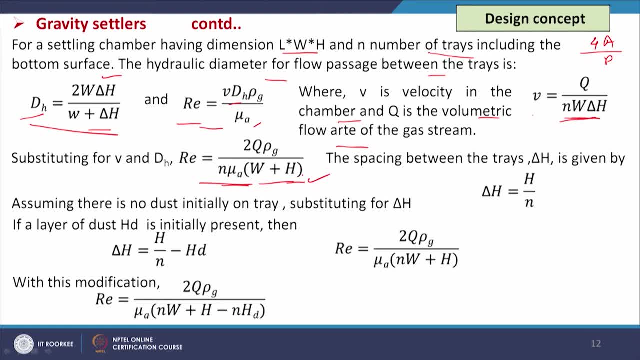 any interval. but if we have some plates and intervals, then del H is equal to H by N, N number of channels. So del H is equal to. again we can get H by N minus HD. if there is no layer initially at the bottom of the any layer, any plate, then HD will be 0, then del H is equal to. 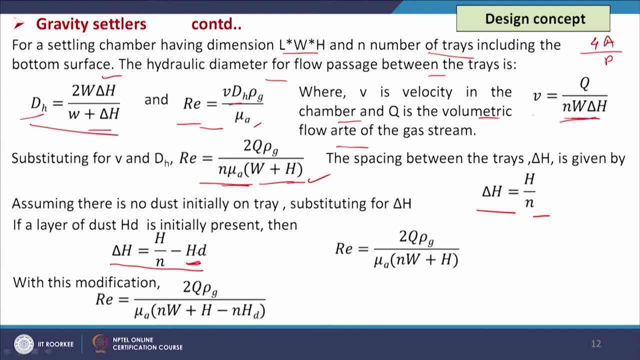 H by N. otherwise this H by N minus HD will be there initially at the bottom layer. there may be some solid in that case. So, Re, we can calculate like this: 2Q rho, G divided by N. Okay, So del H is equal to H by N minus HD, divided by mu A into N W plus H, and with this modification, 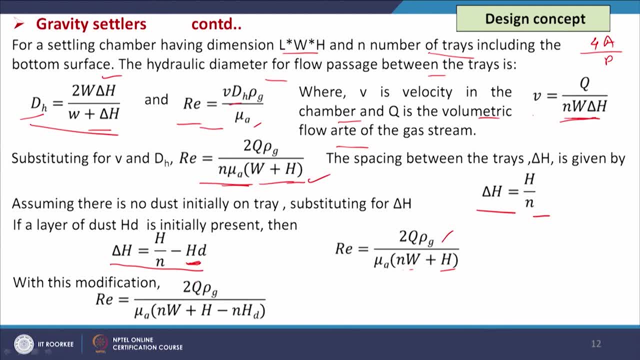 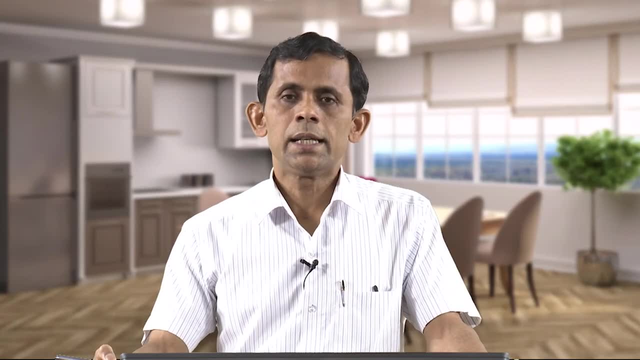 of this del H is equal to H. by N minus HD, we can get Re equal to 20Q rho G into rho A, into N W plus H minus N HD. so these are the expression we can get. Now we are assuming that the flow is laminar, but in reality it may not be laminar and it 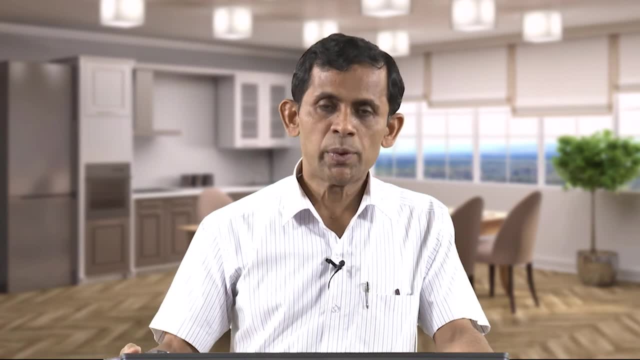 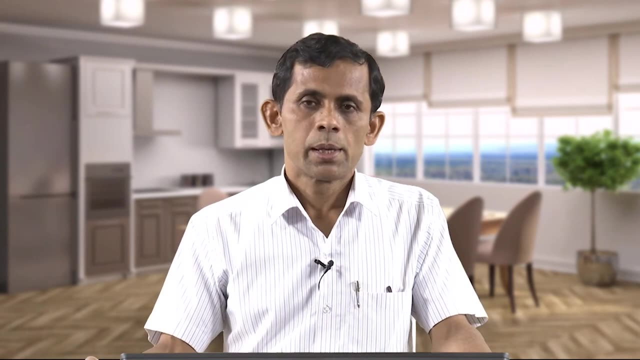 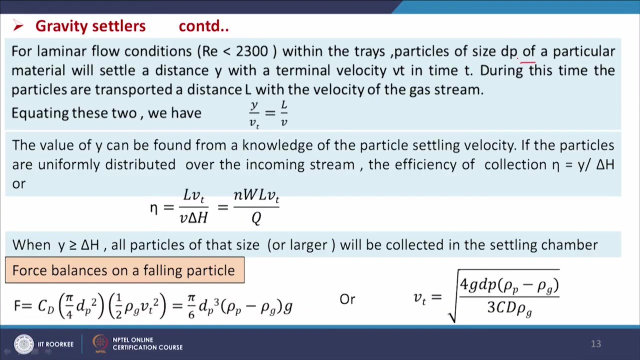 is very difficult to be laminar, So, which we are assuming, that will not, these expressions will not hold good and there needs some modification. So for laminar flow conditions within the trays, particles of size dp of a particular material will settle a distance y with a terminal velocity vt in time t. 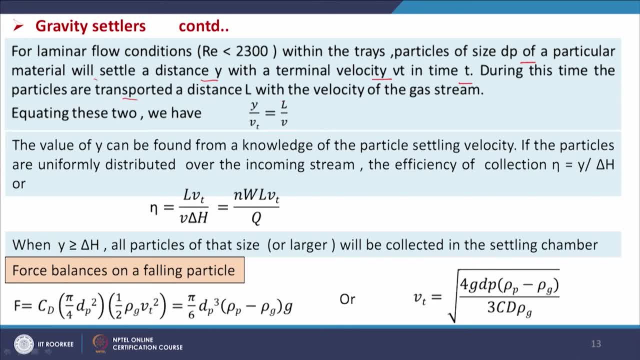 During this time the particles are transported a distance L with the velocity of the gas stream. So y by vt is equal to L by Vt. Okay, Similar expressions we have also had in the previous slide. So y is replaced by capital H in that case. 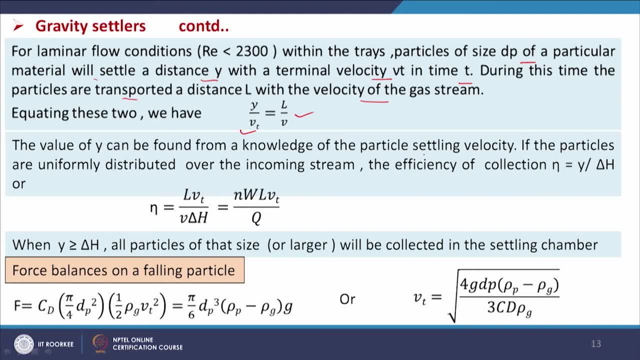 So now the value of y can be found from a knowledge of the particle settling velocity. If the particles are uniformly distributed over the incoming stream, the efficiency of the collection, that eta, will be y by del H. That is very interesting equations or assumptions. 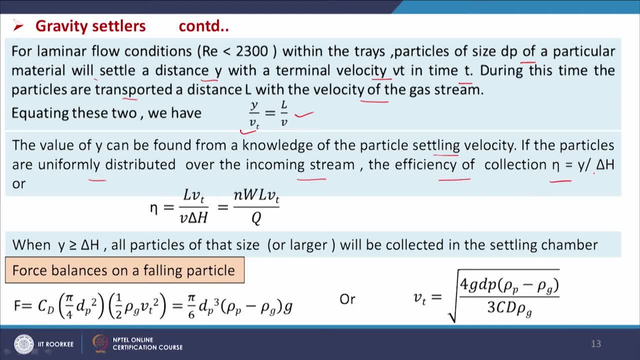 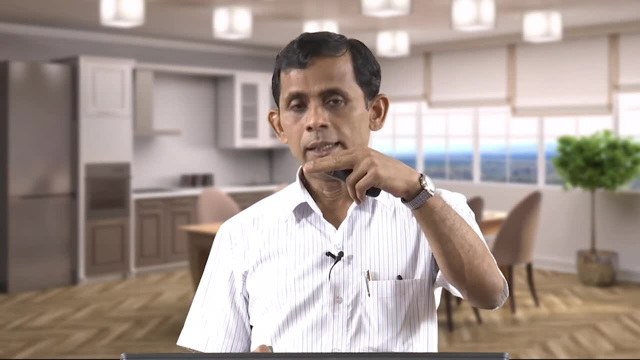 Okay. So say, number of particles are there and it is falling vertically, So from the bottom. initially maximum height is H and then it is falling. Okay, So when the particles are at the bottom, that will be certainly removed, but those particles at the top may not be able to come to the bottom. 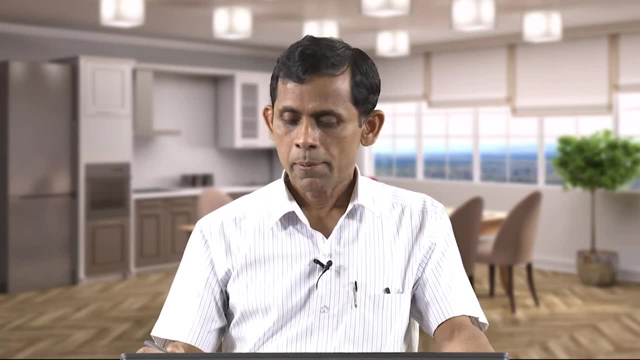 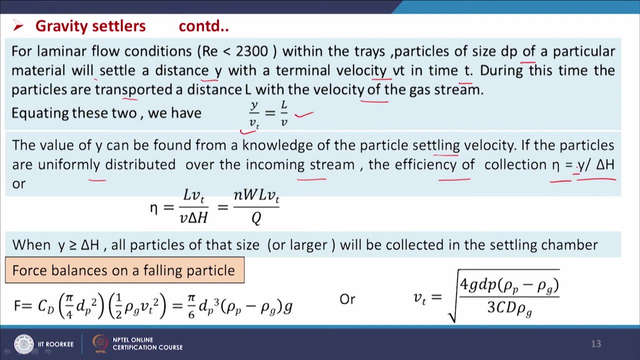 So may not be removed. So efficiency is depending upon the this term del H term, Okay, And the y value, Okay. So the distance through which the particle will travel during this time, So that y by del H, this value is your efficiency. 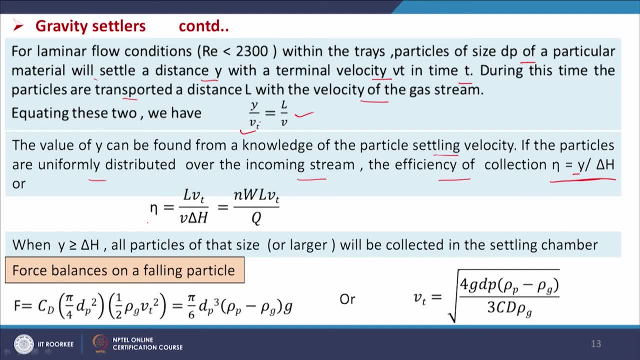 So now, efficiency is equal to y by this. Now, from this expression we can get y equal to L Vt by V. So now, if we put it here, so then we will be getting L Vt by V del H, Now again Vt expressions we have. 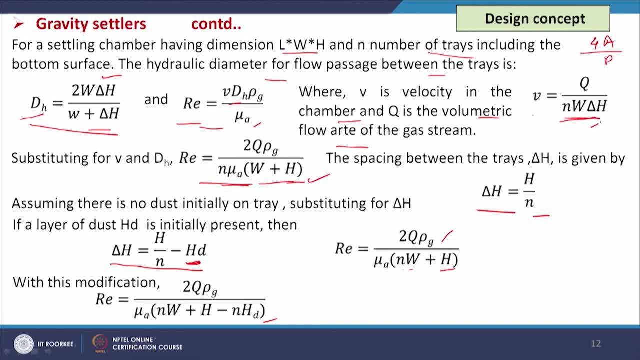 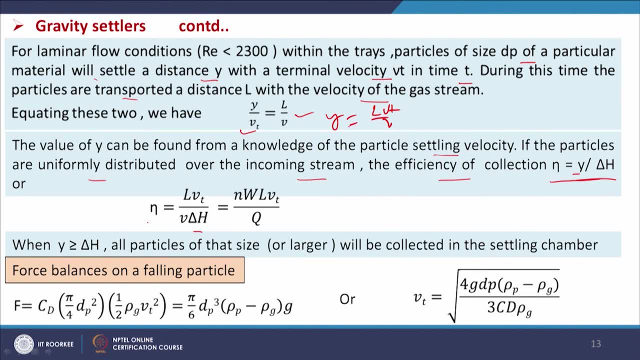 We have this expression: Vt is equal to: Okay, This is our V, And we have Vt is equal to y into V by L. So if we replace that Vt value, then eta will be N, W, L, Vt by Q, Okay. 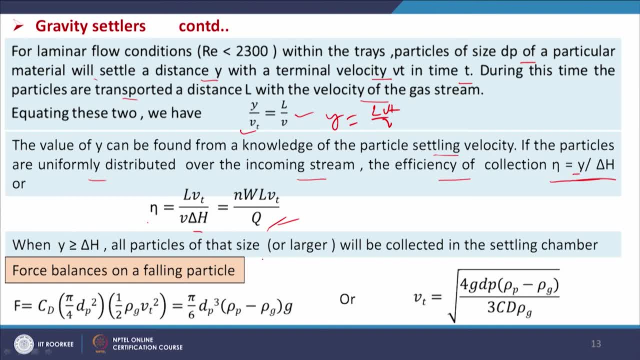 So when y is greater than del H, then all particles of the size or larger will be collected in the settling chamber. And the force balance already we have discussed That. Vt is equal to: Okay, This formula, That is equal to root over 4 g, dp, rho p minus rho g by 3 c cd rho g. 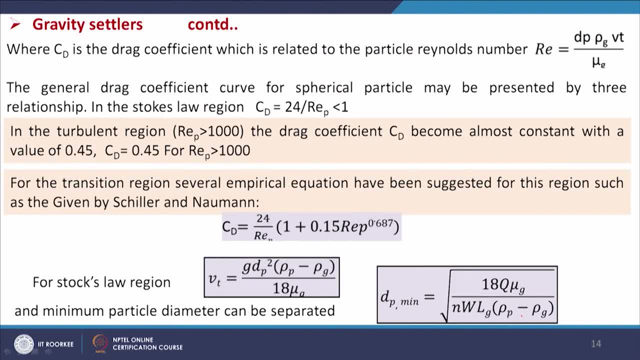 That is cd, That is your suffix, cd rho g And where cd is the drag coefficient which is related to the particle Reynolds number And particle Reynolds number rho d V by mu, So dp. rho g Vt by mu g. Okay, Now the general drag coefficient curve for spherical particle may be present in this. 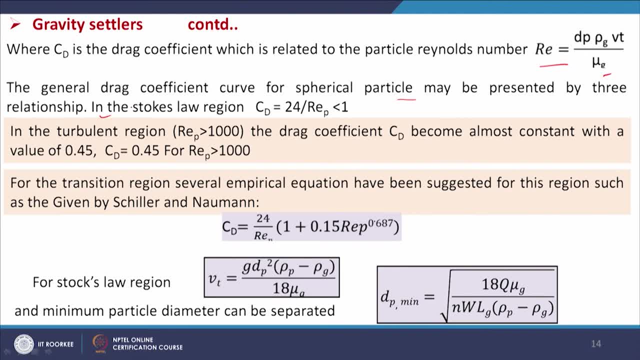 article may be presented by 3 relationships. If we see the drag coefficient, so drag coefficient value will change with the Reynolds number. If it is a laminar flow, then Reynolds number is less. So in that case cd is equal to 24 by Rep. 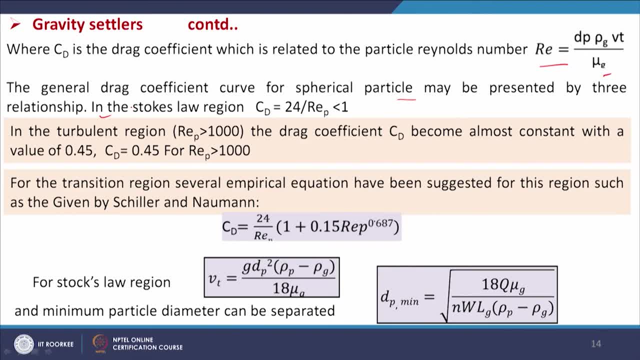 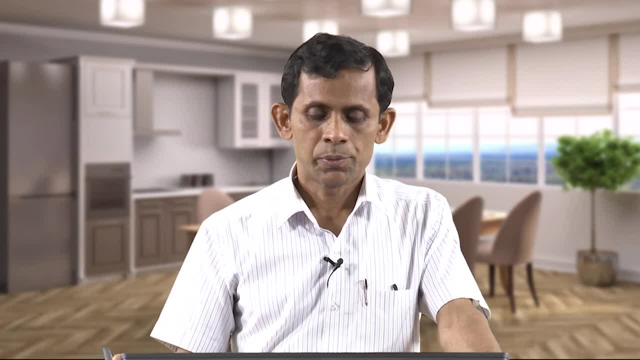 When Rep is less than 1. And when the turbulent region, that is, Rep greater than 1000, then again cd is equal to 0.45 or somewhere it is 0.44.. Okay, So that is the general drag coefficient. 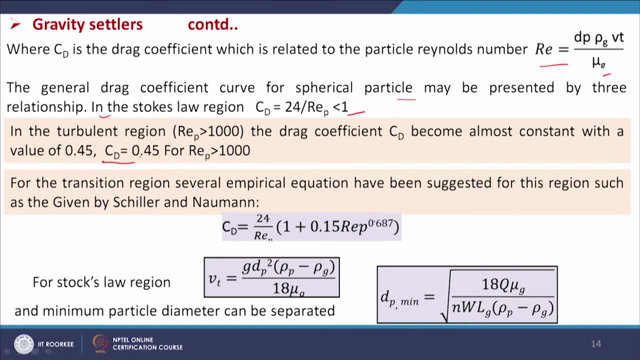 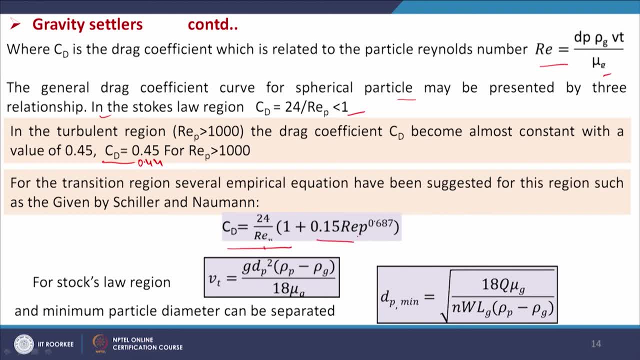 has to be multiplied by some factor, that is 1 plus 0.15 Rep to 0.687.. So if we consider Stokes law, so Vt is equal to gdp square rho p minus rho g by 18 mu g. And then what is the minimum practical drag coefficient? 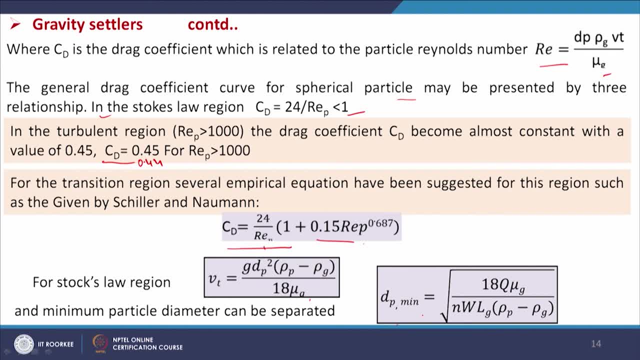 Okay, Okay, minimum particle diameter that can be separated from this expression, we can get dp square equal to 18 mu vt divided by g, rho p minus rho g, that is equal to dp square, So dp root of this. so dp will be root of 18 mu g v t divided by g into rho p minus rho g. Now, 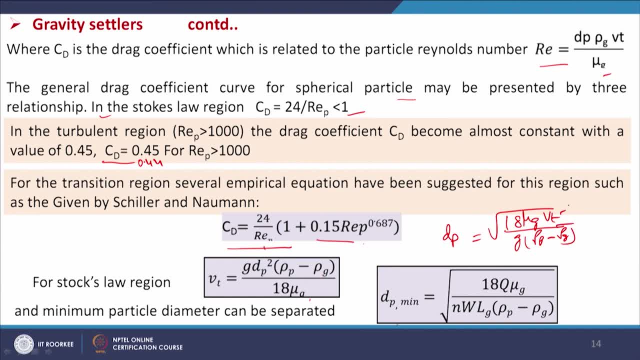 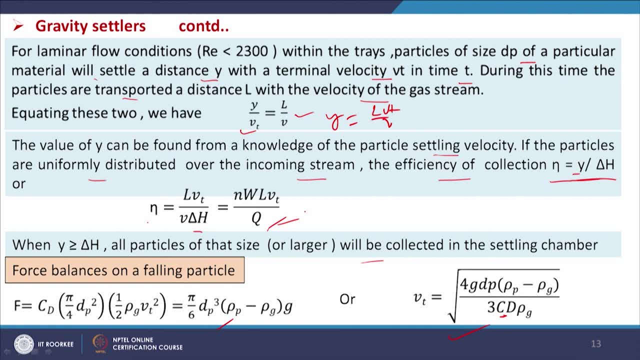 this v t expressions. if we replace then v t, we have got here So this Vt. so you see, V t is equal to this, equal to eta q divided by n w l. So V t equal to eta q n w l. So this we will put this: 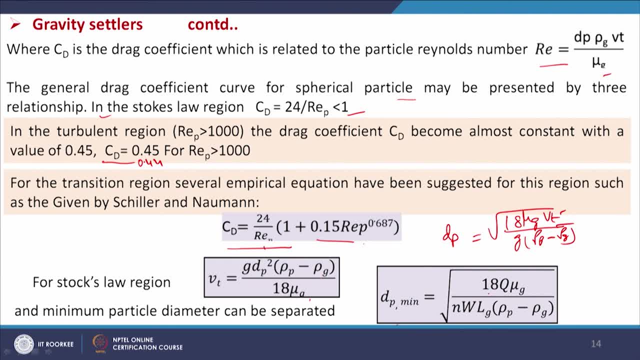 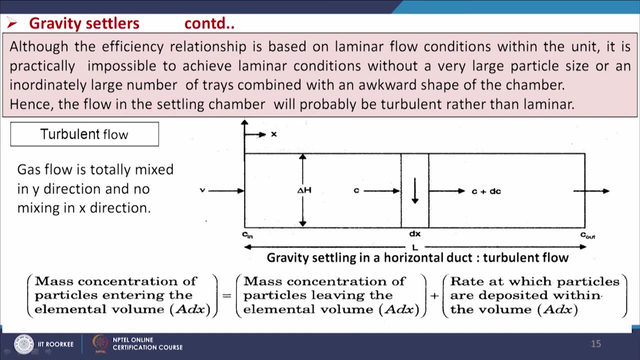 here and we will be getting the expression of V t, minimum, 18 q, mu, g, n, w, l g, rho p minus rho g, because in this case eta is equal to 1.. So that is why we are getting this expression Now, although efficiency relationship is based on laminar flow conditions within the unit. 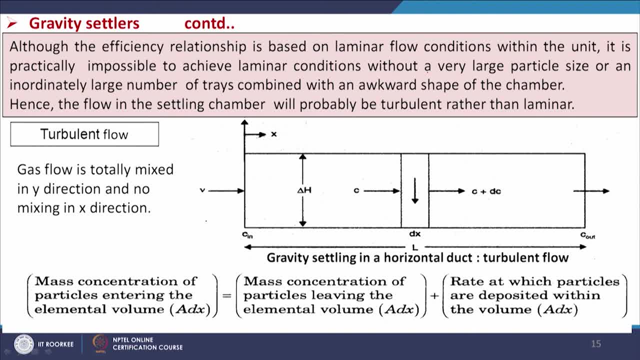 it is practically impossible to achieve laminar conditions, So there will be some turbulence, So there will be some variation, as you have mentioned. Now let us see: we have the velocity of the gas stream as v and it is going through this chamber and we are considering a small 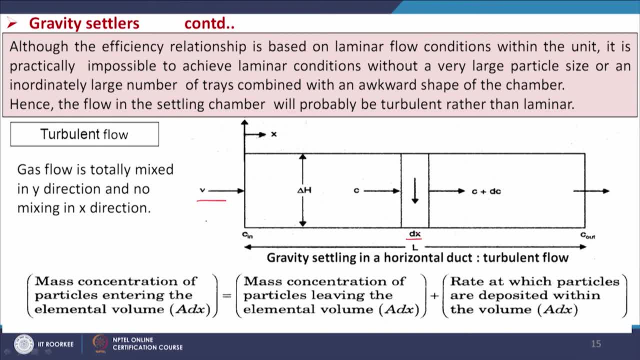 volume and this is the distance, dx. So in this case, if we get the mass balance, So the mass concentration of particles entering the elemental volume that is equal to A cross-sectional area into dx, and this volume and mass concentration of the particle, leaving the elemental volume ADX, okay, So these are related like this. 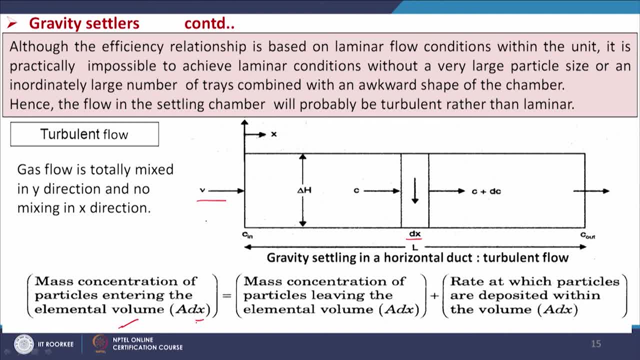 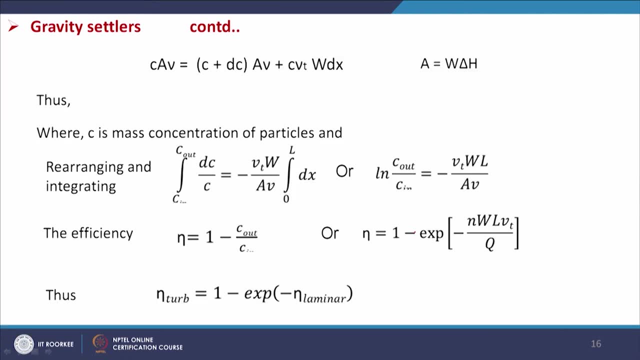 mass concentration of the particles entering the elemental volume ADX, equal to mass concentration of particles leaving the elemental volume ADX plus the rate at which particles are deposited within the volume ADX. So this is the mass balance of the particles. So the first term we are getting A into V, into C. So A into V is the volume into C. 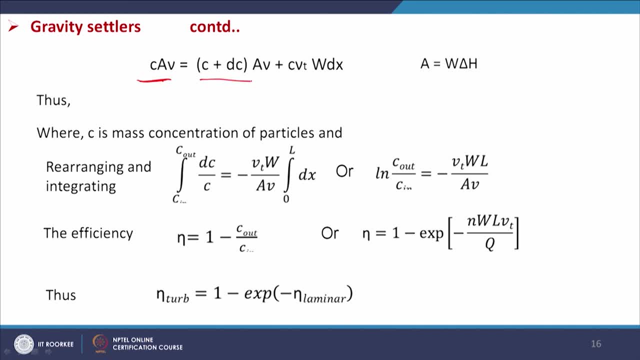 So this is the concentration total mass and similarly, for this is outgoing, that is C plus DC. here we are getting C plus DC concentration. we have to multiply it by the volume. So volume is the concentration of the particles, leaving the elemental volume ADX plus the. 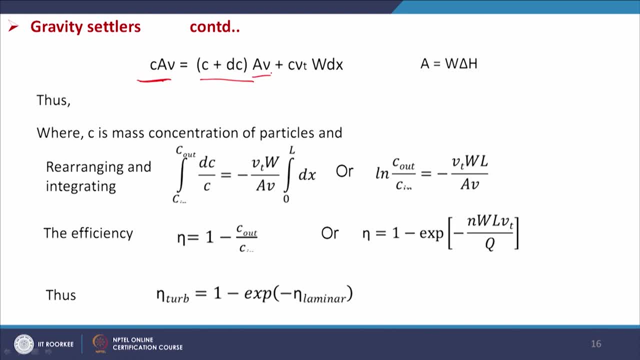 volume is equal to what: A into V. So for the same case, in this case the volume is nothing, but we are getting W into dx, into Vt, because it is falling in vertical direction. So C into Vt, into W, into dx, where A is equal to W, into del H. So now, from this expressions: 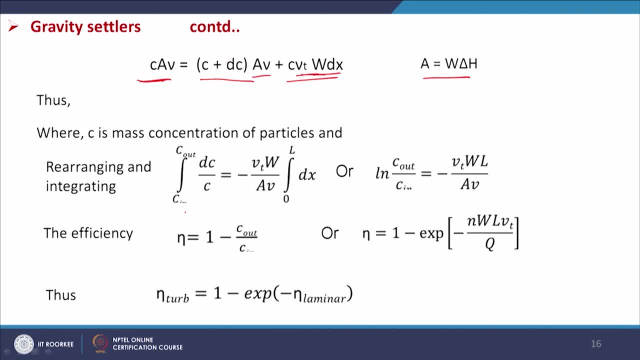 if we integrate, then the expression will be like this: C in C out, DC by C, equal to Vt, into W by Av into 0 to L, dx or L n, C out by C in equal to minus Vt, W, l by Av. Now if I want, 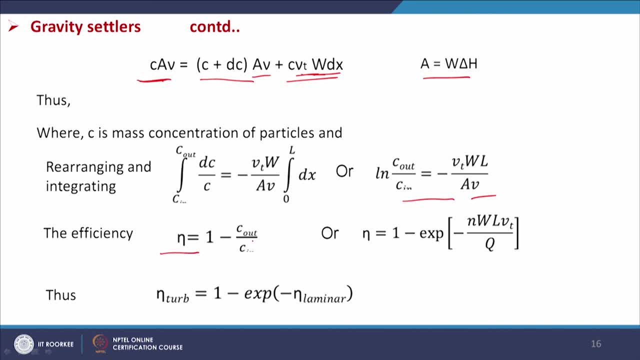 to get the efficiency. So efficiency is equal to nothing but 1 minus C out by C in or C in minus C out divided by C in. So L n C out by C in is equal to this expression we are getting. So C out by C in will be your exponential of minus Vt W l by Av, as mentioned. 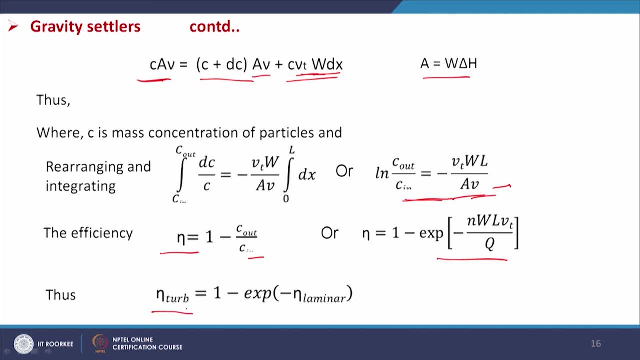 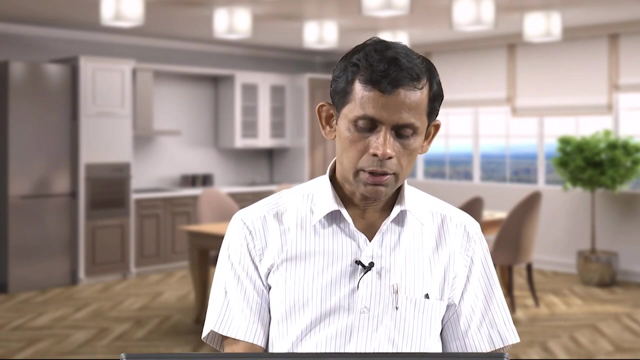 here, in case of turbulence, efficiency will be 1 minus exponential of minus. this N, L, W, V, T by Q. but this is nothing but the efficiency at laminar condition. So laminar conditions if we can find out the efficiency of collection that can be converted into turbulent conditions. 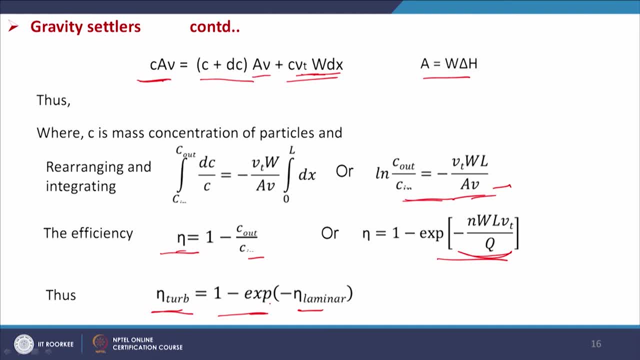 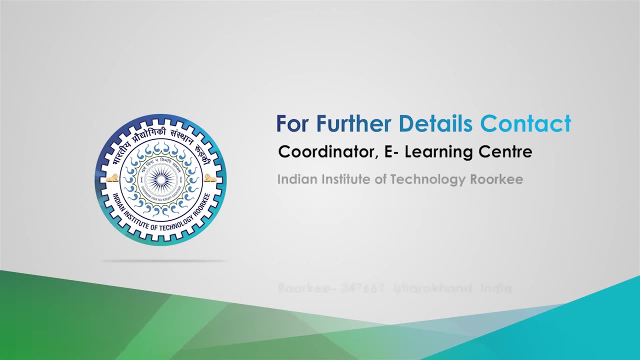 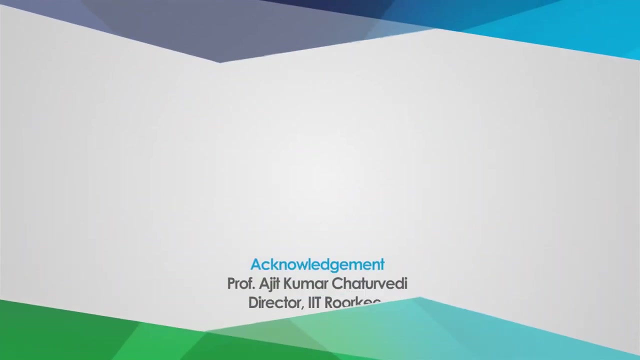 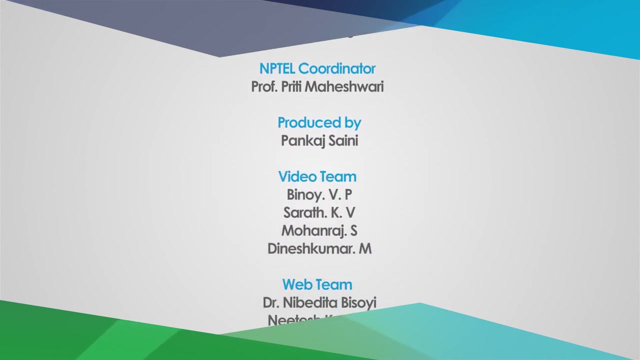 by using this expression. So these are the different mathematical expressions which can be used to calculate the efficiency for the separation of the particles up to this in this class. Thank you very much for your patience.